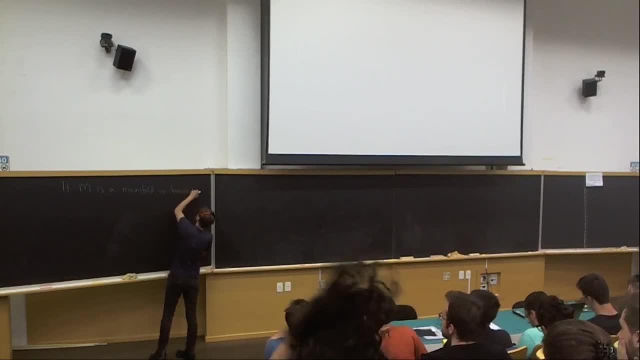 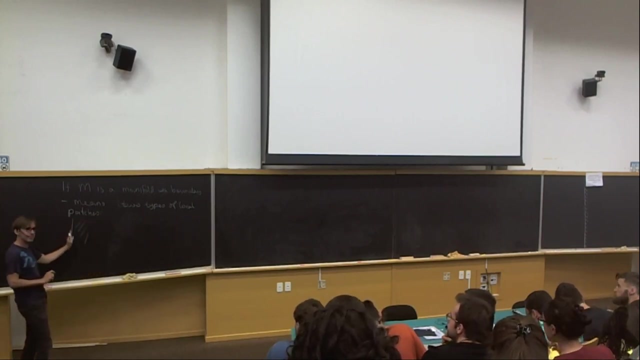 which means there are two types of local coordinate patches. So here's what your manifold might look like. It has some boundary. So there's two types of patches. One type of patch lies in the middle. One type of patch is given by. we have coordinates y1, yk which are in some ball. 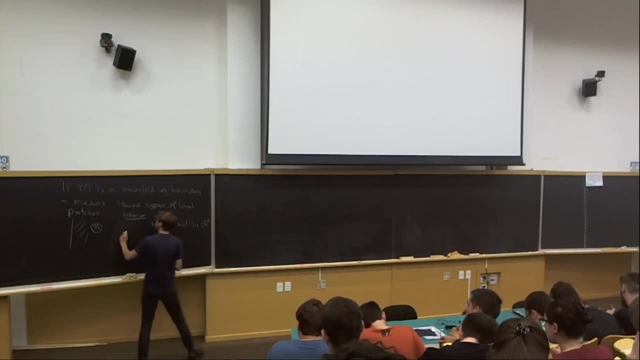 And there's also boundary patches- y1 to yk, as before, But now we take y1 to be non-negative and the boundary is when this is equal to zero. So this guy with y1 to yk which live in some ball, except that this guy is non-negative. 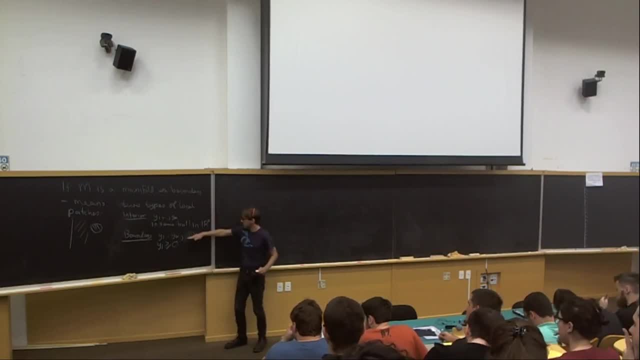 so this patch looks like this: Some kind of half Half of a ball describes a region which includes the boundary. So if m is orientable and k and you also want- it's a kind of technical remark- you want it to be compact so that the integral converges. 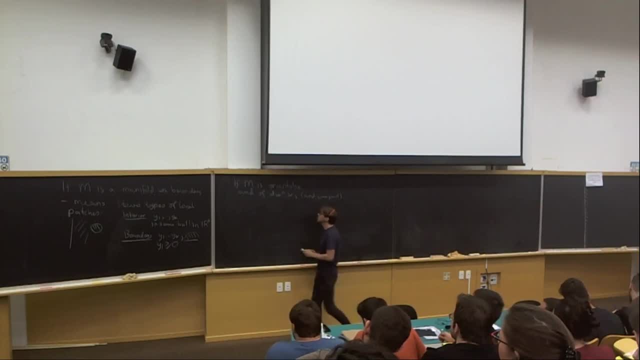 but let's not worry too much about that. If you don't know what that means, then we can integrate. We can integrate a k-form over m Just in the same way we did before. we just divide it up into patches, do the integral in each patch. 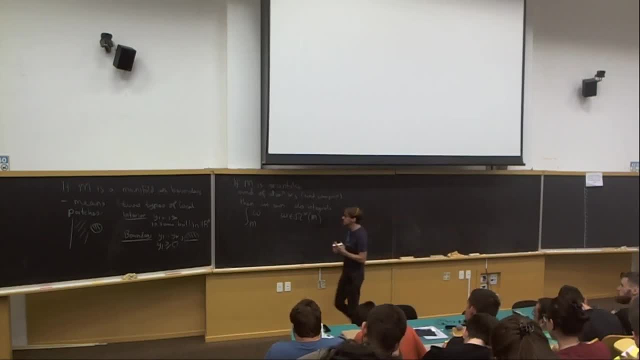 Notice that change of coordinates on the local patches doesn't doesn't affect the integral, because the change of coordinates picks up a Jacobian factor. So what Stokes' theorem says is is that the integral over m of the deram operator applied to a k-1 form. 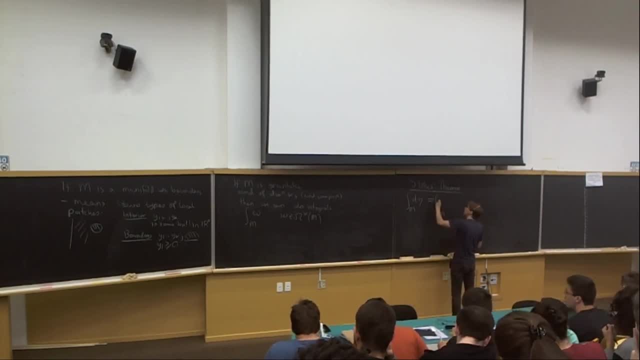 is the integral of the boundary of m of the k-1 form of the k-1 form. Okay, so this is kind of a familiar kind of statement. It's a much cleaner way of writing things that applies uniformly to all manifolds and all dimensions than what we saw in dimension 3.. 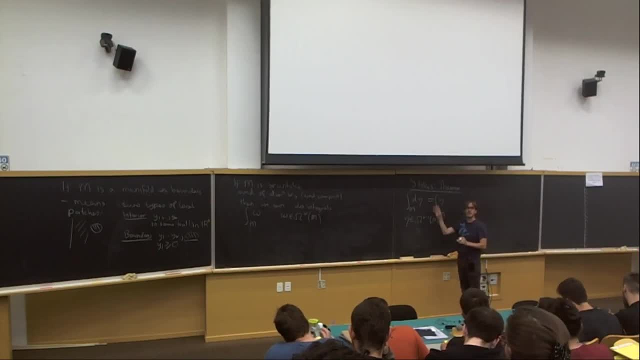 In dimension 3, when you were dealing with surface integrals, it got a bit kind of nasty with how do you write this? you know You had all these. uh, I don't know. it seemed a bit confusing to me anyway. 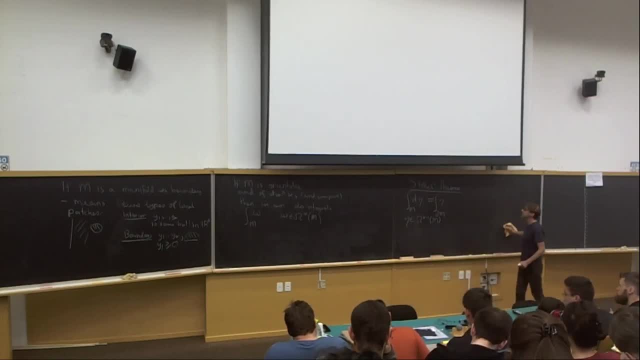 the traditional way of writing it in dimension 3.. So how do we prove this? So let's divide m into cubes Like this, Like this, And it's going to continue in most directions, but I'm drawing it so that here is the boundary of m. 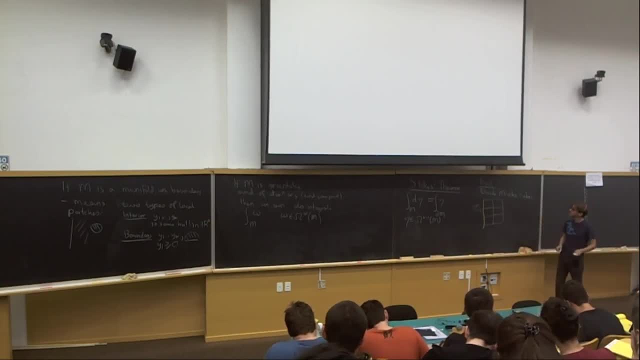 Okay, so we're cutting our manifold up into cubes and most you know, in the interior each cube is surrounded on all sides by other cubes, but on the boundary one side of the cube is left open And each cube is oriented. 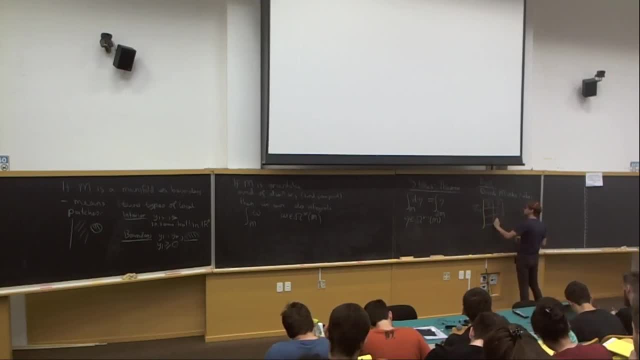 so I'm drawing it in dimension 2, so there are squares, So our manifold has a consistent orientation, so I can draw an orientation on each square in this case, and they kind of match up when they are joined by a face. Now the integral of my form. 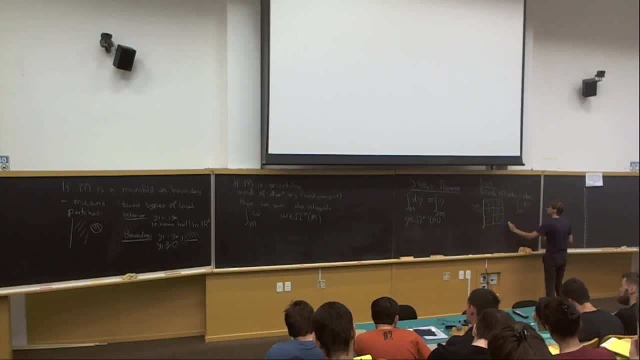 is equal to, you know, the sum over the cubes of the integral, over the cube of the form. This is one way to define the integral. And now what we're going to do is say: well, we know, if we have just a cube in flat space, 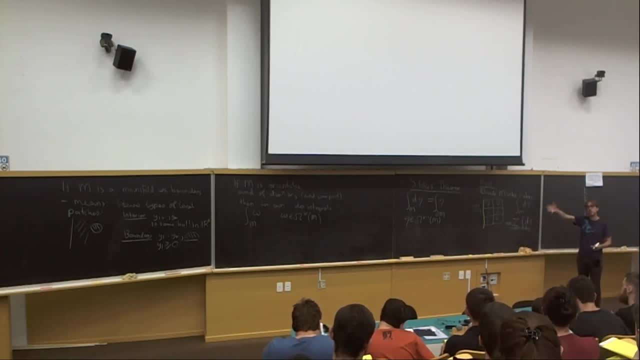 the integral of a total derivative will be the same as the integral or the sum of the integrals of all the faces. This is just the ordinary facts that the integral of a total derivative picks up the boundary. So the integral over a cube. 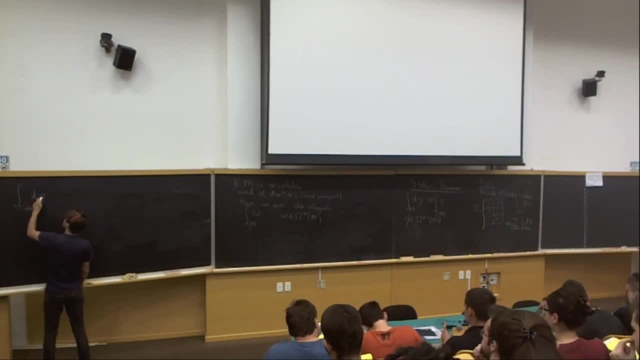 of the total derivative is the same as the integral over the boundary of the cube or the sum over the cube of this form, just by usual rules of integration. So we might think, since we're summing over all cubes, we're going to get a crazy number of boundary terms. 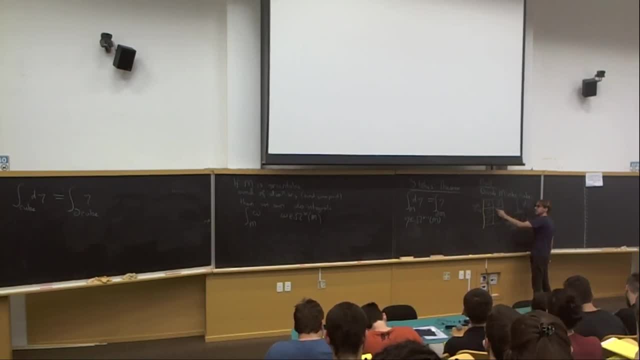 We'll get. this boundary term will appear as a boundary of this cube, but it will also appear as a boundary of this cube, and so on. So we'll get all these boundary terms, but what we'll find is that most of these boundary terms cancel. 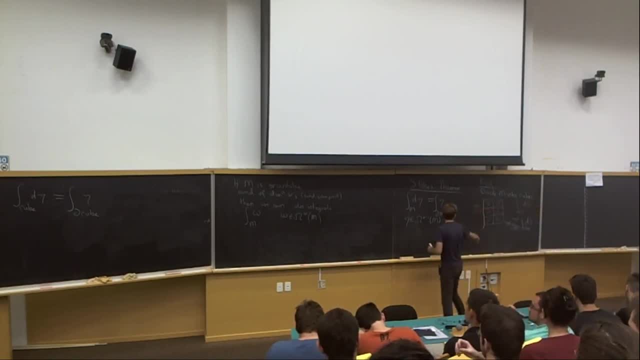 except the ones on the boundary, on the boundary of the manifold here. So each k minus one dimensional face of M which is in the interior here, will contribute twice. So I have a k minus one dimensional face in the interior. 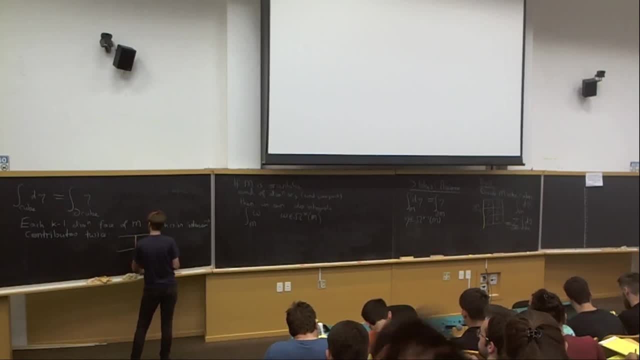 here, I'll dot it in pink. It contributes once from the boundary of this cube and once from the boundary of this cube. So what we want to show is that these cancel, And the reason they cancel is that they contribute with opposite signs. 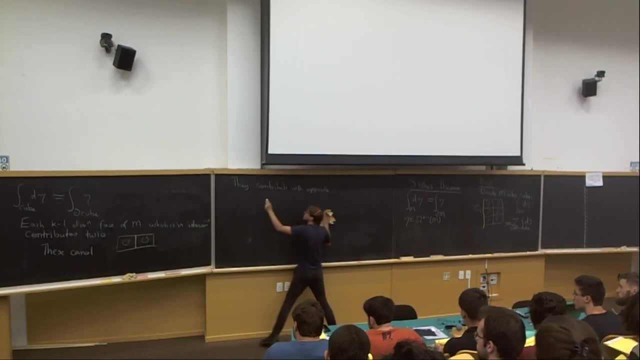 So let's see why this is true by kind of pulling them apart a little bit. So when I take the boundary of this square, I pick up the boundary integrals going in that direction. So when I take the boundary of this square, I pick up the boundary integrals going in that direction. 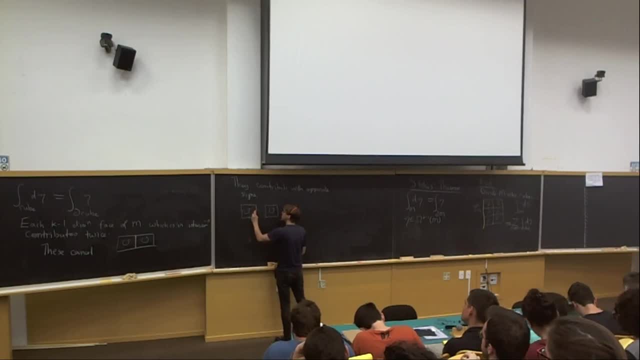 So, in particular, this pink face will get a, will be integrated in that way, Whereas this one, it's also going clockwise, but it will give you the integral in the other direction. So they just cancel. So I've drawn this in two dimensions. 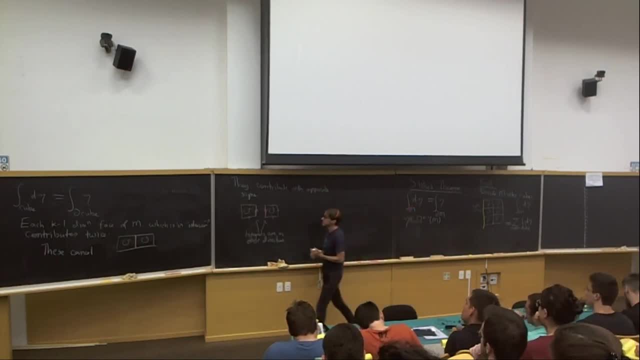 but a similar argument applies in an arbitrary number of dimensions. Now, the only faces which don't get cancelled by this procedure are the ones which have square only faces. So the only faces which don't get cancelled by this procedure are the ones which have square only faces. 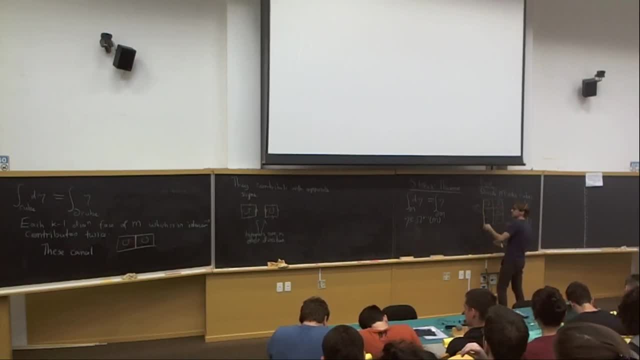 And what's actually going to happen is that the integral itself, it's only on one side. There's nothing on the other side to cancel that integral. So we're just left with, so the sum over the faces of the boundary of M of the integral of eta. 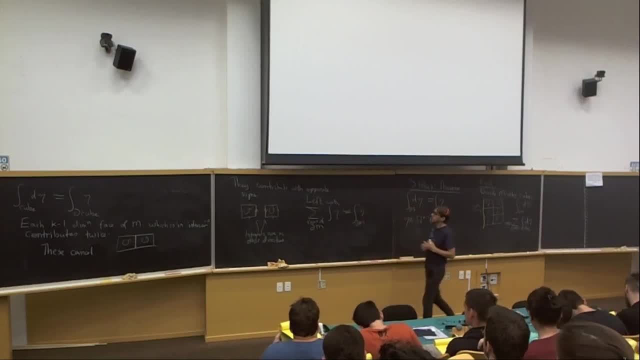 not that, it's just the integral over the boundary of M, this formula. So there's some nice yeah question. So I think that the concept of pullback is kind of a bit confusing to people, but it's nothing mysterious, right. 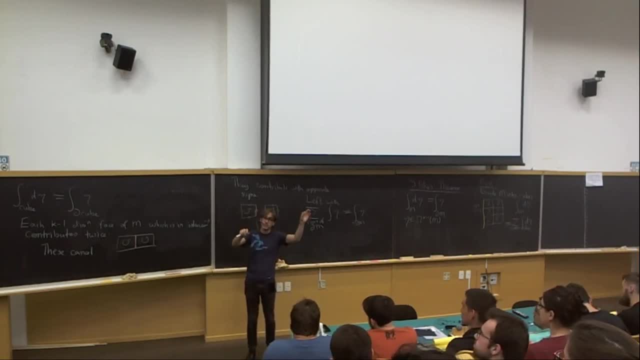 When I have a function and I integrate it, I only care about the values of that function on the region I'm integrating. What the function does at some faraway points doesn't matter. So the pullback of a differential form is just taking your differential form and looking at what it does on that region. 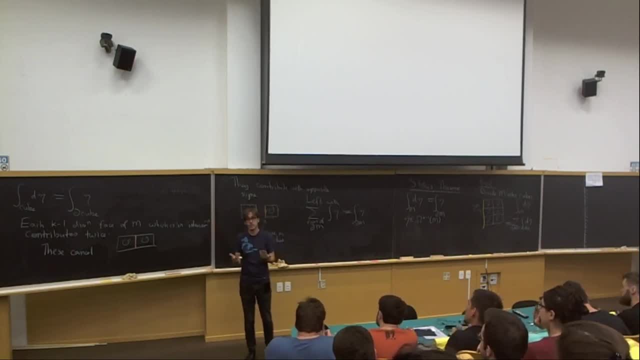 because that's all that's going to contribute to the integral. So that's all it is. Yes, yeah, that's a good way to say it. Yes, so because we're defining, we're saying that a coordinate patch on the boundary lives in a half space. 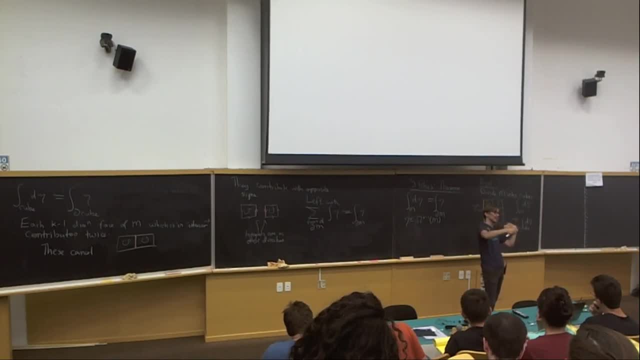 So it always has one of the coordinates non-negative, So it never touches the other half. So even if there are different coordinate patches, they all live in the same half space. Does that answer your question? Okay, so there's some kind of fun things you can derive from this. 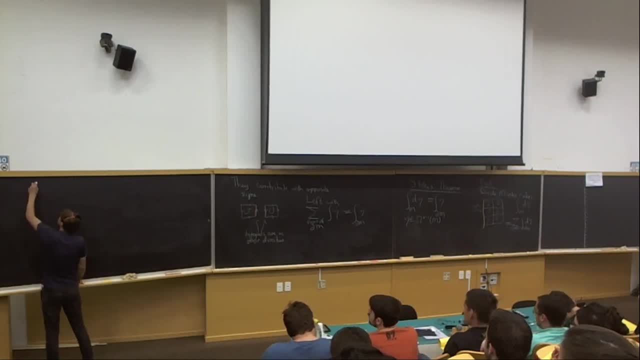 So here's one. So Suppose we have is an n-dimensional manifold and y is an oriented k-dimensional manifold, and y is an oriented k-dimensional manifold and y is an oriented k-dimensional manifold and omega is a k-formant m, which is closed. 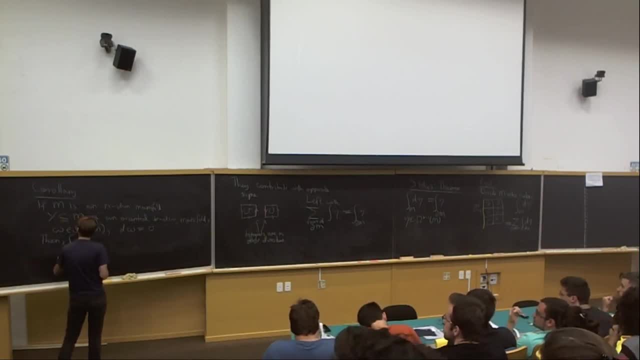 Then the integral over y of omega doesn't change if we vary y. So this statement is just like the statement people are familiar with from counter-integrals. So why is that, If we have one parameter: family of submanipoles, of submanifolds? 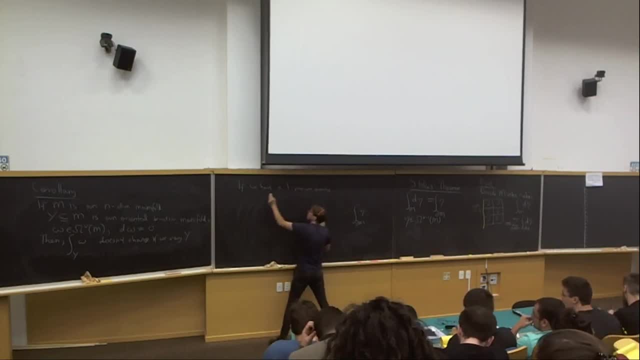 of submanifolds yt, where y0 is equal to y. then I'm just going to describe intuitively what's happening. So this is y0, and over here is some kind of wiggly thing, it's y1.. As I vary y, they, 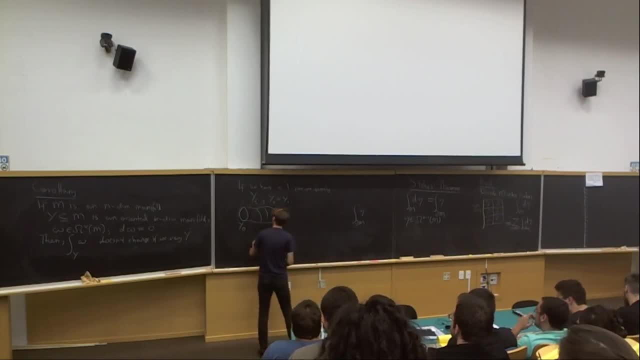 sweep out a cylinder. This is a cylinder with boundary, say y hat, where the boundary of y hat is y0, union, y1.. So then, the integral of d omega over this cylinder is the integral over the boundary of the cylinder of omega. The boundary has two pieces. One piece is the y0, which is 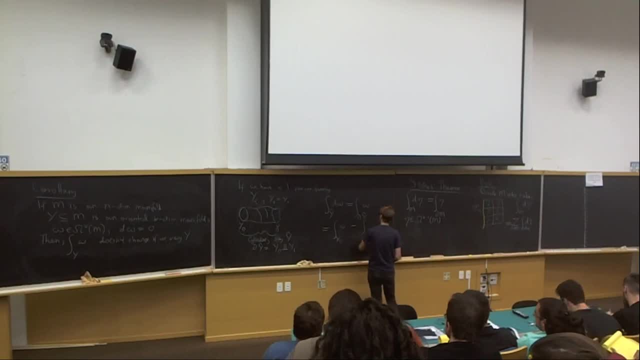 what we originally started with. and the other piece is y1.. So you might ask, why is there a minus sign? Well, the minus sign is because of the orientations. We have, y, as some orientation say. y goes that way. 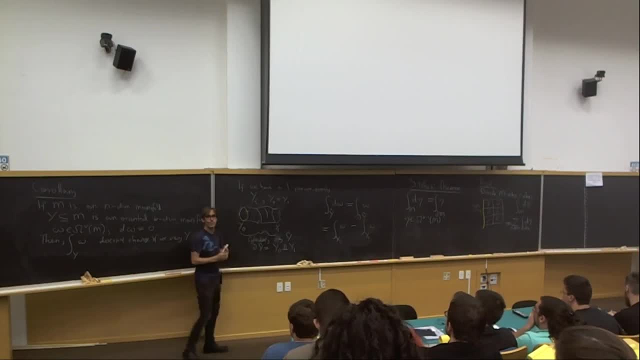 I have to orient the cylinder. maybe I orient it that way And then, because this arrow points in at one end and out at the other end, this one must go that way. And just in the same way, the line integral, the contribution of the endpoints. 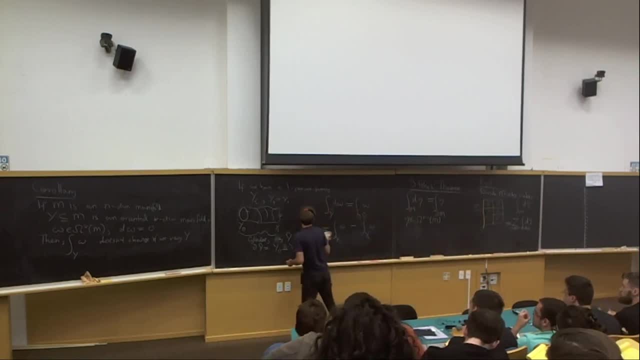 is a different sign, it's the same thing. So here's a kind of fun example of this. Suppose I have a region in the complex plane, An f z z bar, a function on u, and then d of f z z bar, d z. 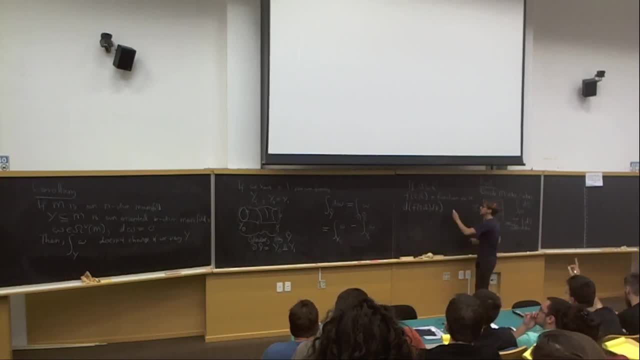 We have this one form: f times d z. Yeah, If we have a one parameter- family- sorry short for parameter, I don't know. So if I have a function on a region in the complex plane, we can take a one form: f times d z. 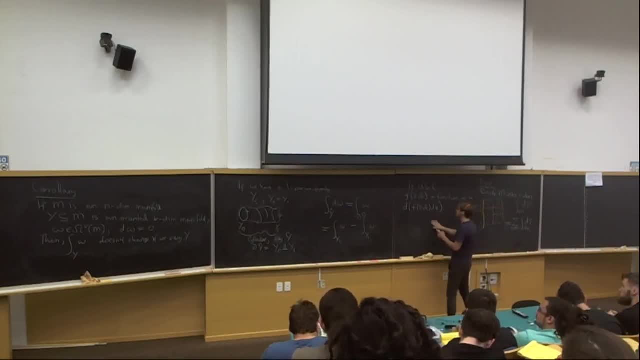 where d, z is d, x plus i, d, y, And you can check that this is closed if, and only if, f satisfies the Cauchy-Riemann equations. So the Cauchy-Riemann equations are of course. 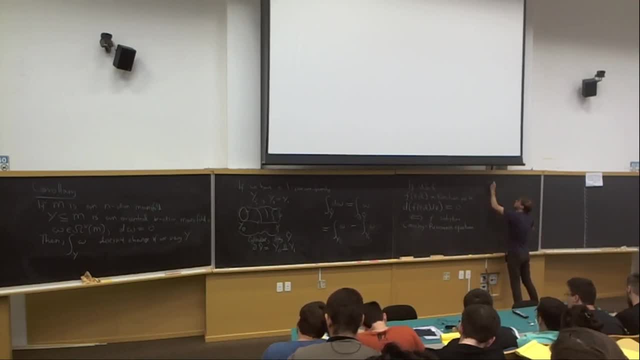 that d f d z bar, which is half of d f d x minus i d f d y, equals zero. So applying this kind of story about how the integral of a closed one form, 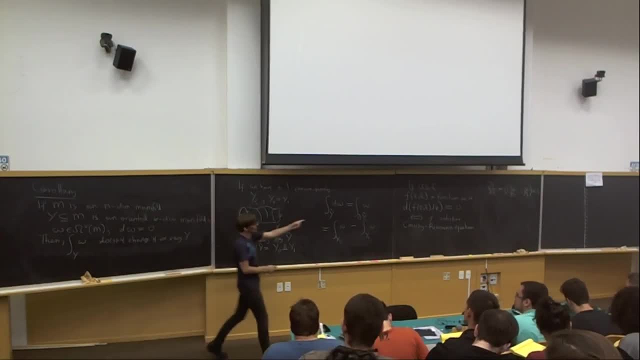 doesn't depend on the contour to these particular closed one forms gives you the usual story of contour integration. So this implies that the integral over a contour is equal to the integral over a contour. So d z doesn't change, It's got. I think it's holomorphic. 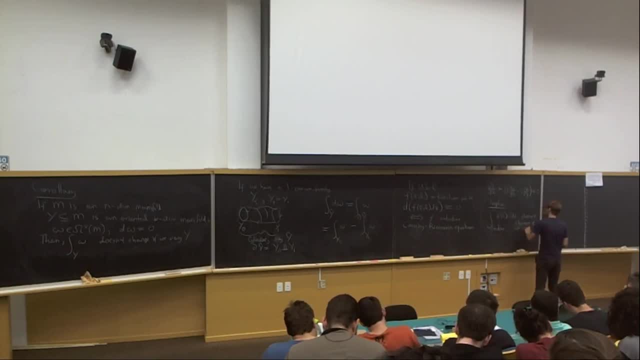 If we vary the contour, All right, Okay, Mm-hmm. Oh, there's only two pieces of the boundary, Because the cylinder I'm thinking of like literally a cylinder, There's two boundaries, One at zero. 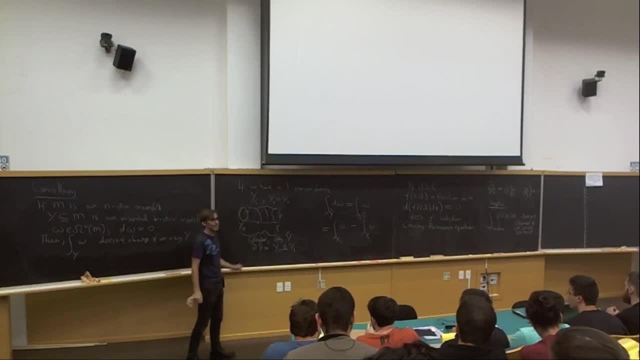 one at one, Two boundary components. So I'm taking my original manifold and moving it along and as it evolves in time it sweeps out something a bit like a cylinder, which is two boundaries: the original time and the final time. In the middle there's no boundary. 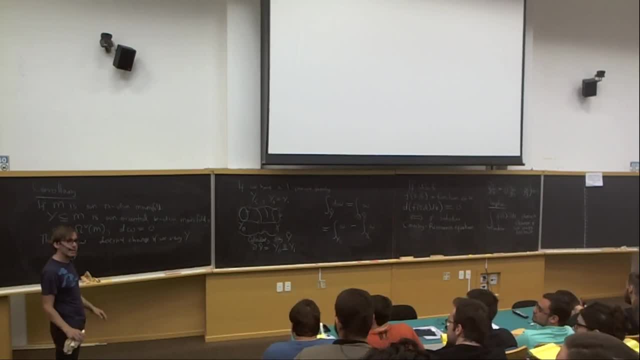 Yes, Exactly, I didn't. you know this was a more math course. Yeah, If this was a math course, you'd have to be very careful about all these things. but yeah, I'm thinking of a smooth variation. So you don't want to change the topology, you don't want to kind of rip. 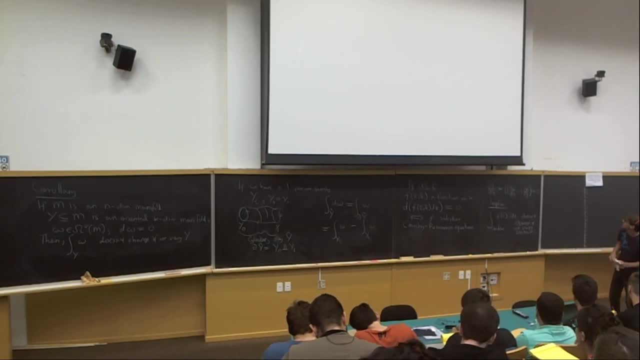 it up into pieces or anything. Okay, So I I haven't explained very much why cohomology is a topological invariant, So I want to spend a few minutes explaining these points and then I'd like to move on to explain, if I have. 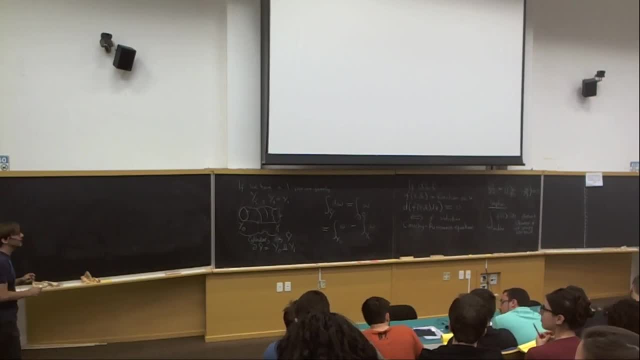 time the connection between the ramp forms and the gate. So if we have two manifolds and a map from m to n, you've seen we've got a map. f upper star takes a k form on m to a k form on n. 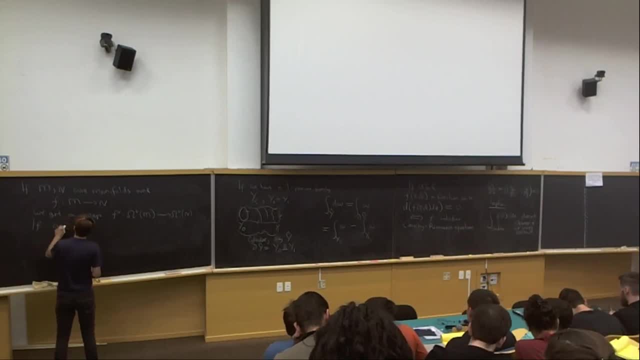 So if I have a closed k form, then we let- I'm going to use this notation- with the square brackets around omega, which is to be the corresponding cohomology class. So yeah, there are some questions about the meaning of these equivalence relations. 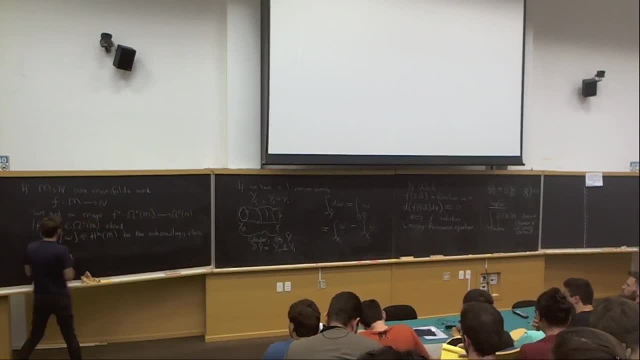 So the way to think about it is, you know, this might be a gate field and this cohomology class is the gate field. This is the gate equivalence class. Adding on d of a k minus 1 form is like a gate transformation. 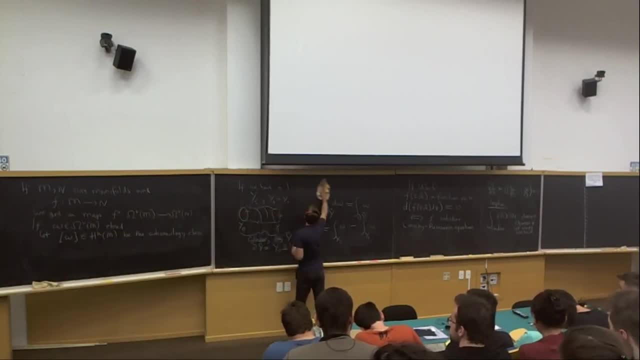 And in fact, if this was a 1 form, it would be literally a gate transformation. Ah, I always make this up, Sorry, Thank you. I always get confused between m and n, So this should be n as well. 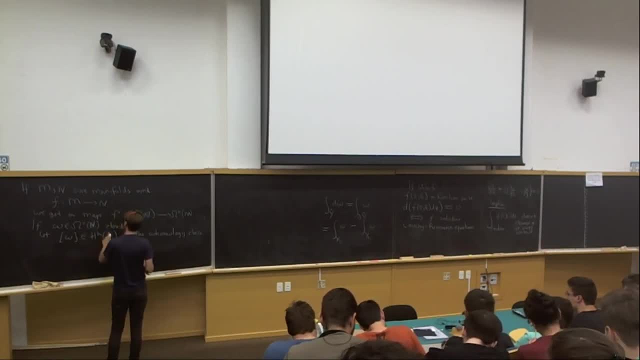 So we can consider f star of omega and this is closed. So we can ask: and it: does This cohomology class only depend on the homology class of omega? And the answer is yes, if I change omega by d of something, by a gate transformation. 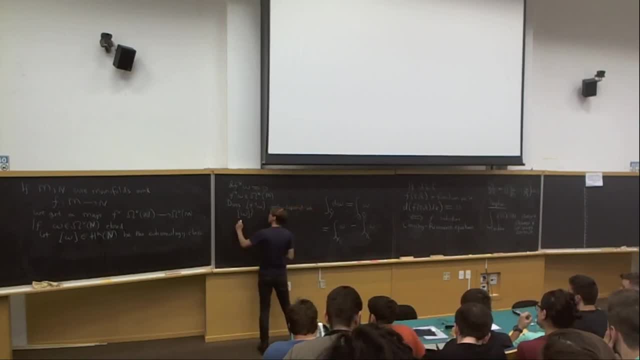 then I also change f star of omega by a gate transformation. So if we change omega by d of something, then I also change f star of omega by a gate transformation. So if we change omega gets changed to omega plus d eta, then f star of omega gets changed. 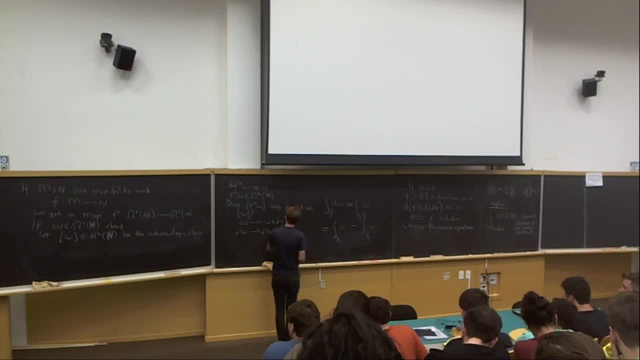 to f star of omega plus f star d eta, which is f star of omega plus d f star eta. So this d of f star eta is like a gauge transformation by f star of eta. So it follows that f star of omega only depends on omega, on the cohomology class omega. 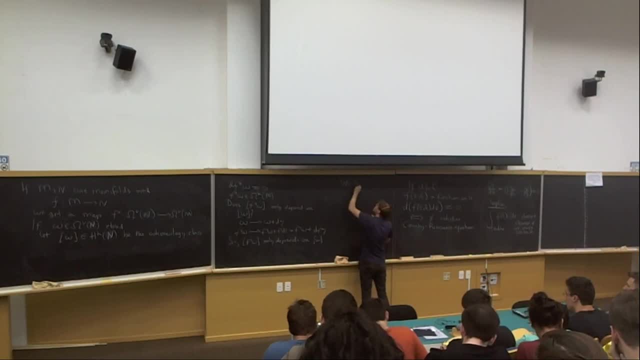 This means that f star of omega we have a map at the level of cohomology, So I'll continue to call it f star. I hope this won't cause confusion. So the first thing that is going to tell us about why cohomology is insensitive to small perturbations. 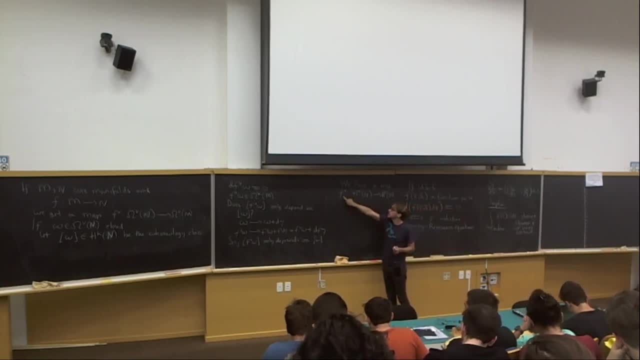 will be that this map does not change. if we've a acabar co-molouge, he does not have… change if we vary f in a smooth way. So if f of t is a smooth… okay, F ofder, When is that normal? 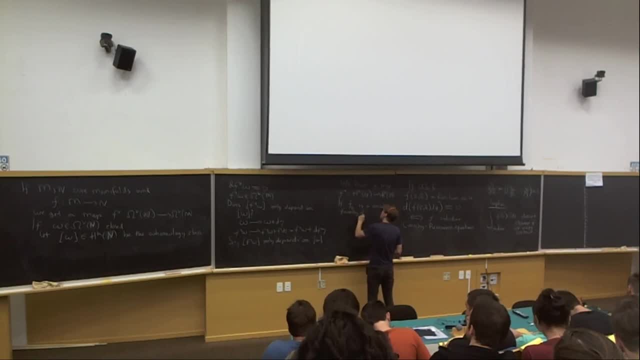 No Ft of maps from M to N, then d by dt of F star mapping from HKN to HKM is zero. So if I have a family of maps and I pull back a cohomology class, then the resulting 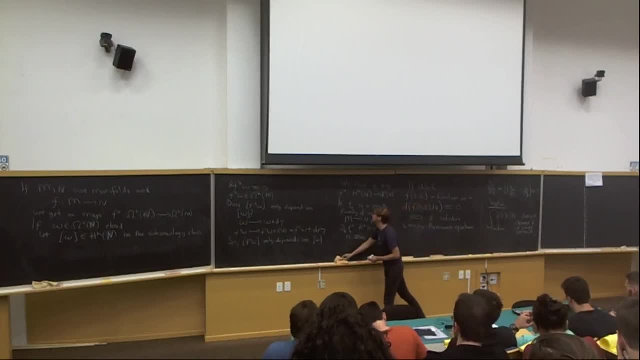 cohomology class does not change as I vary over this family. So why is this? Let me quickly give you an example. This is an important statement which is worth remembering, but let me quickly give a proof of this statement. The proof itself, maybe, is not so important. 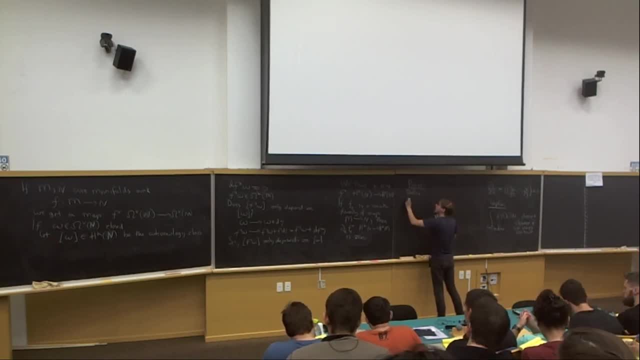 We define F hat which goes from M times time. Well, I don't know, we'll see To N- by F hat of M. comma t is F lower T of M. So there's a. we're saying we view time as a parameter in the map. 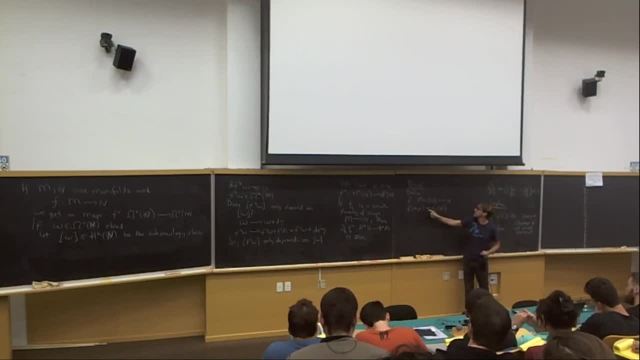 It takes a point in my manifold times time to the value of this one parameter family of maps at that point. And then we write, and we can write, I can pull it back using f hat, and this will have two pieces, one of which is just 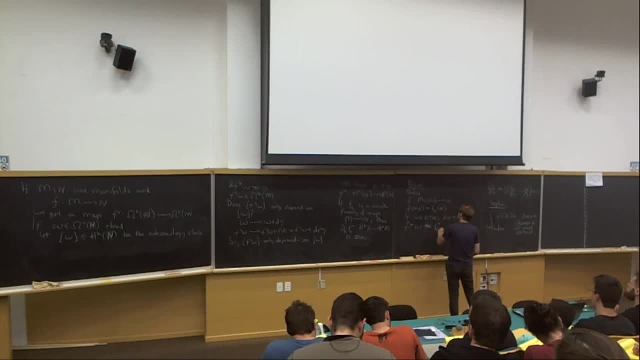 the pullback using this one parameter family of maps and the other of which is just something else which depends on dt. so here what we're saying is: well, this is some form on this manifold, so there's a piece which has a dt and a piece which has no dt. 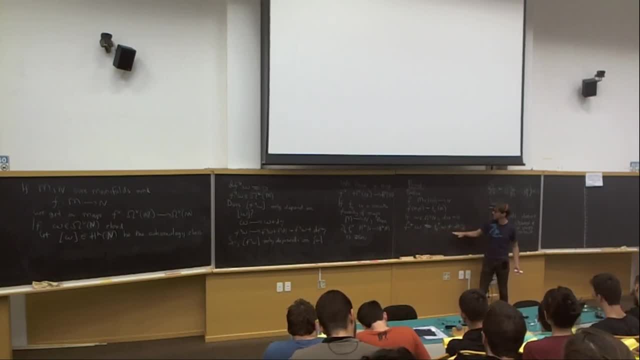 we're writing it as a sum of the piece with no dt and the piece with one dt. now, d f, hat star omega is equal to zero, so so I'll probably have to go a little faster, so maybe don't worry if it's on, do you clear? 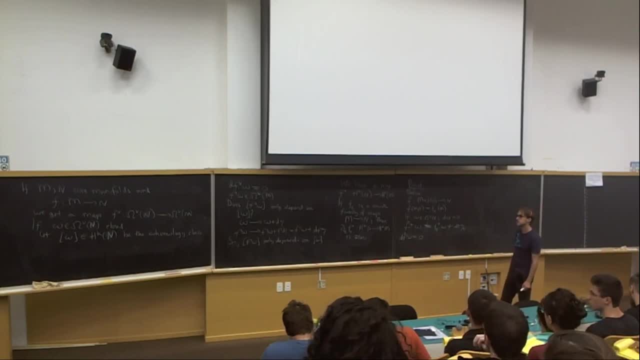 yeah, here, this one, this one, this is meant to be a little omega is a form. it's in capital, omega k of n is that? oh no, I really meant. I really meant this because I want to. Yes, it's essential that this is zero. 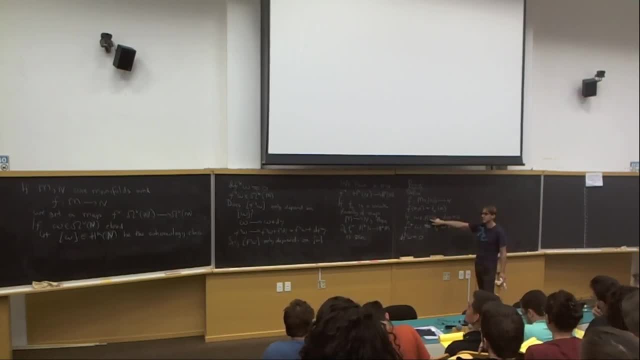 And I don't want to pass to cohomology quite yet. I'll do that at the end of the argument. So let's just look at what this equation says. This equation has two terms. It'll have a term which involves a dt. 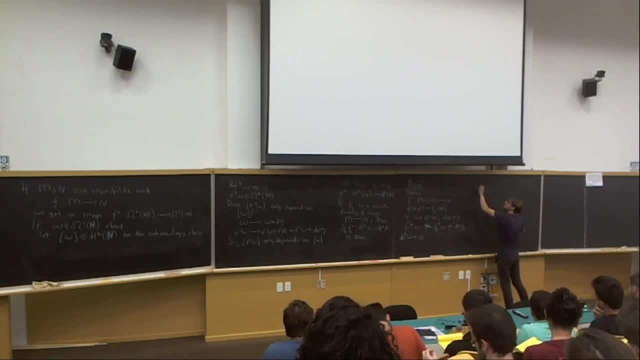 and which does not involve a dt, So d f hat star of omega will have a term which is like d on m, the derailleur operator on m plus dt del t plus. this is actually a minus for sign reasons, so we're just using the fact that the derailleur operator 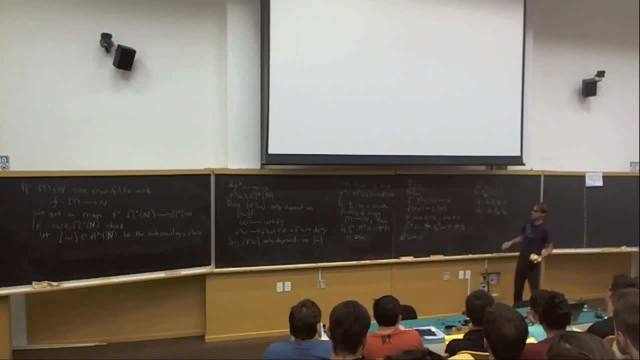 on. this manifold is a sum of the one here and the one here, So this argument is really too technical, maybe for this course. Now, let's just look at the various terms and we'll set everything to zero. So this piece doesn't have a dt. 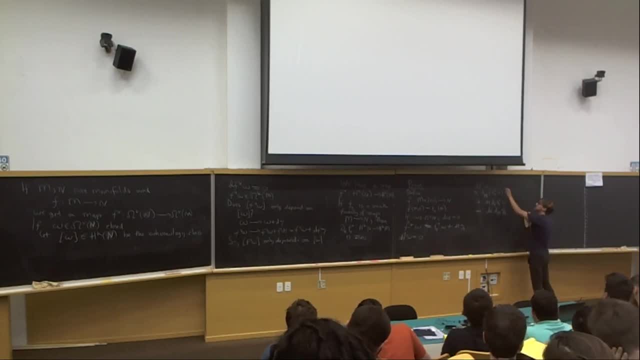 so this guy must be zero just by itself. So this piece is zero And this piece, this is the sum of two pieces, each of which has a dt, So these must sum to zero. So we conclude that the variation, if I differentiate with respect to t, 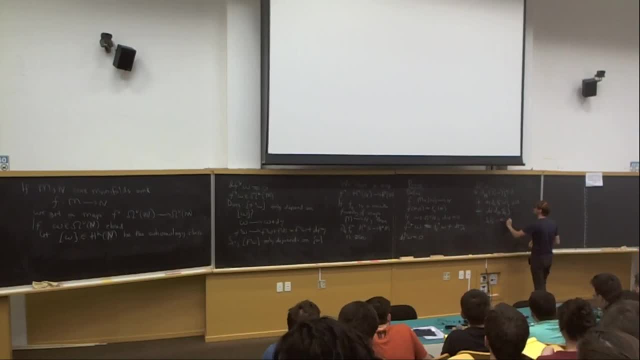 what this family of things looks like. it is that a derailleur operator applied to something, Therefore the cohomology class. well, that's the formula we're going to use here. It doesn't change. Hmm, It's. I haven't told you what it is. 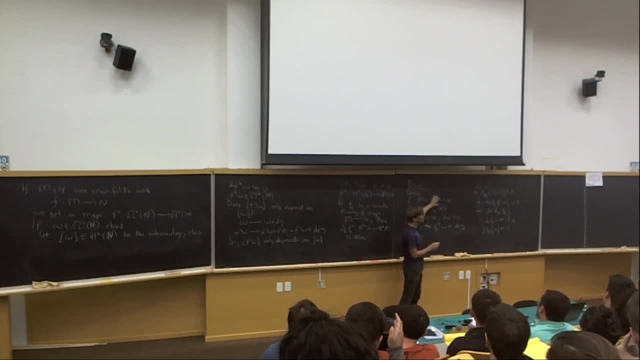 I mean, I'm just saying, whatever this guy is, it's a form on this manifold and let's expand it. It'll have a piece with no dt, which is this, and a piece which contains a dt, but I'm just calling it a t. 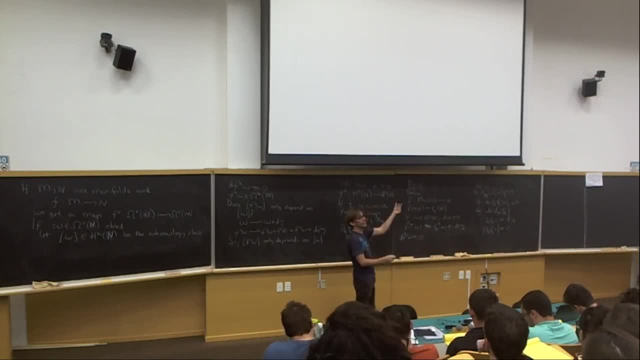 I haven't given you a formula for it or anything like that, It's just we know there must be something like that. Okay, so this kind of slightly technical argument tells us that this operation on a cohomology doesn't change if we vary the map. 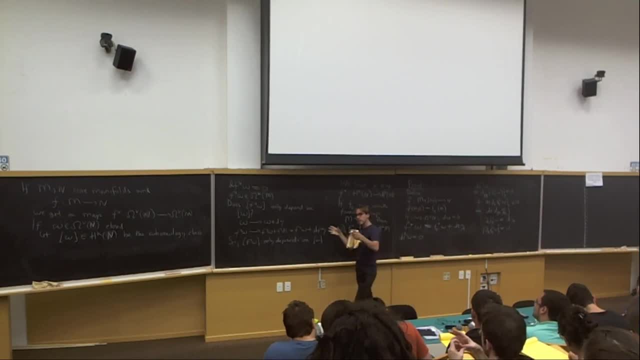 This is really similar to the kinds of things we were discussing earlier. You know, if I vary a contour, the integral doesn't change. It's a very similar situation, Because integrals can be defined in terms of the pullback on cohomology. 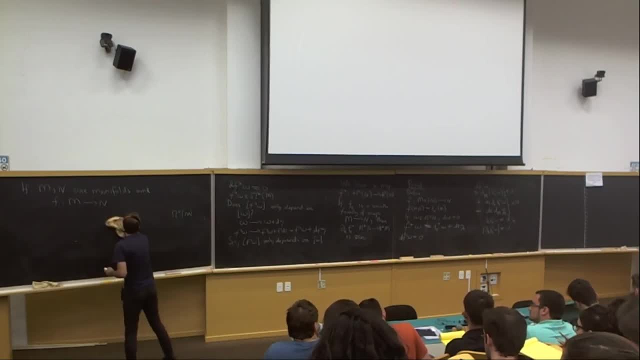 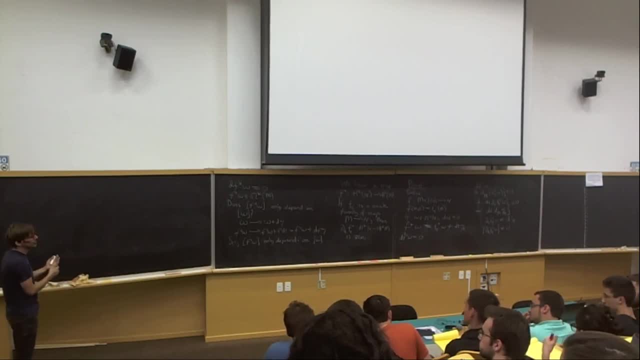 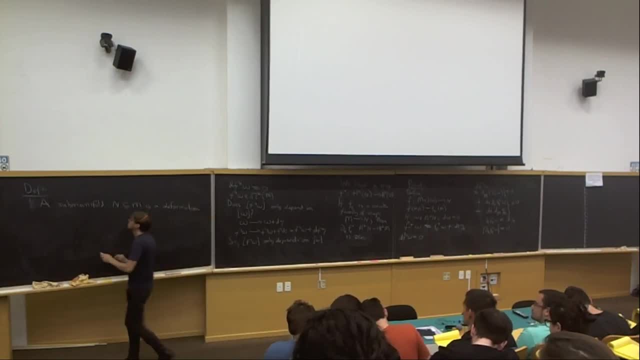 But if there is a one-parameter family of maps, Ft from M to F, we're at the following properties. So firstly, Ft: if I take a point in N, I get back that point in N. Secondly, F0 of any point gives me back that point. 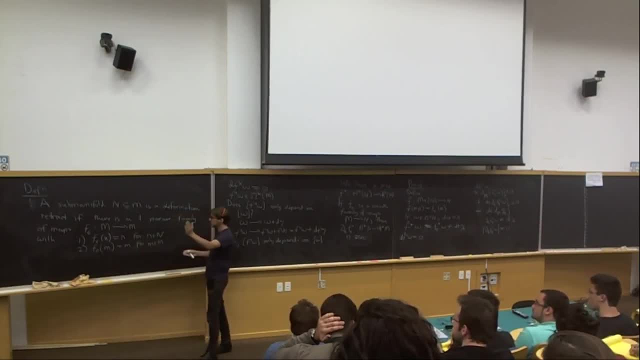 So if I take this family of maps, T equals 0, it's just the identity mapping, it does nothing. And as I move it along, the third property tells us that F1 of any point is in N, So at T equals 0, it does nothing. 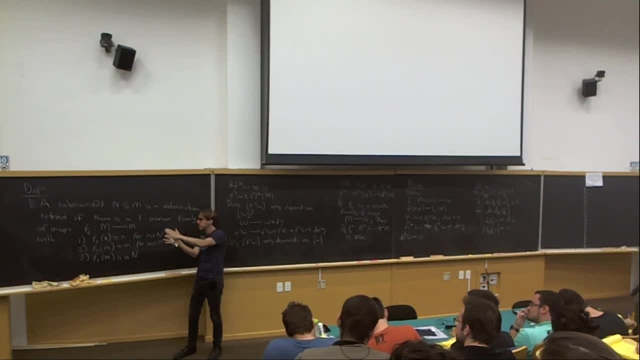 And as I increase T it squishes things down until eventually everything is squashed down to this submanifold. So Kind of picture to bear in mind might be a circle living inside a cylinder, And my one-parameter family of maps just kind of squashes everything down to the middle. 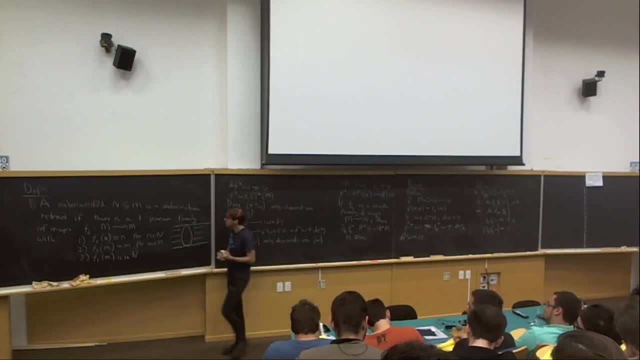 Like that. So being a deformation retract like this, it is a very common thing to see. So So well, mathematicians would say they have the same topology, They have the same essential topological features, These little kind of fuzzy fuzzy things that one can squash away. 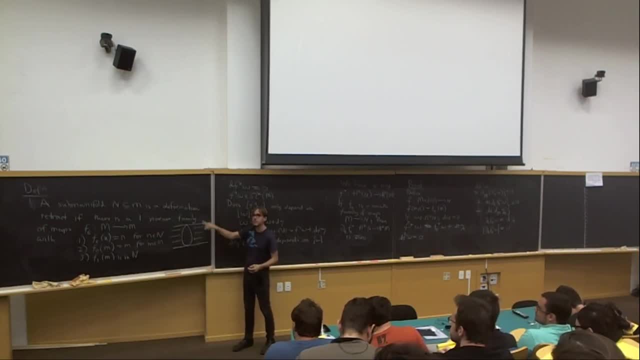 they're not important. This cylinder, this circle in the middle can't be squashed away. But all this kind of nonsense over here is not important for the topology. 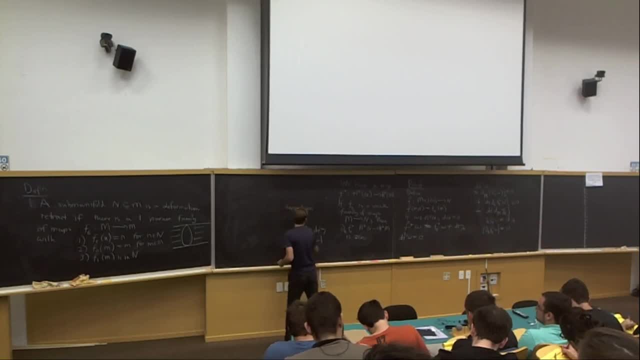 So here's some examples. So if I take the origin in Rn, so this is the deformation retraction. So this is really easy to see. We just define ft of x to be 1 minus t of x. Then when t 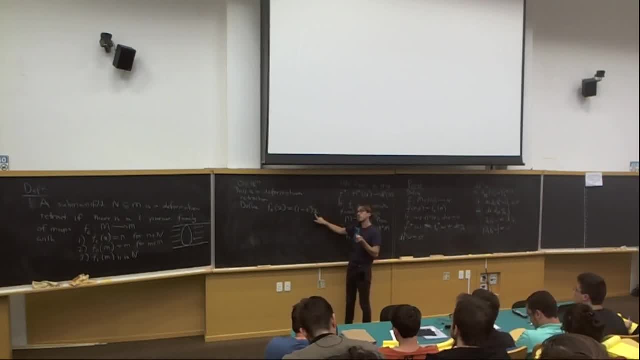 is 0, I just get back what I started with, and when t is 1, I go back. I'm squished down to the origin. That's very simple. So if I take the sphere, This is also a deformation retraction. 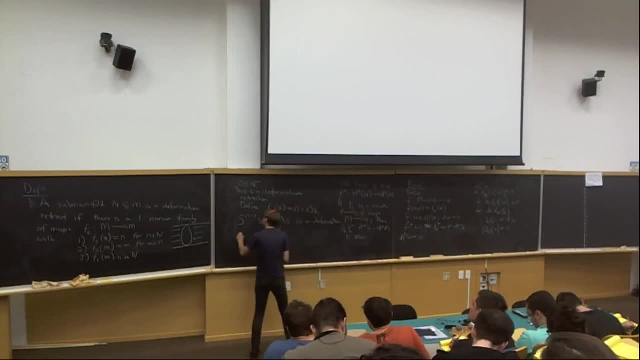 So how does this work? We define ft of x. So the intuition would be: I take a point in this space, This is okay. I could take the second point in the space. You just make 2 times one or this and seed it to be two. 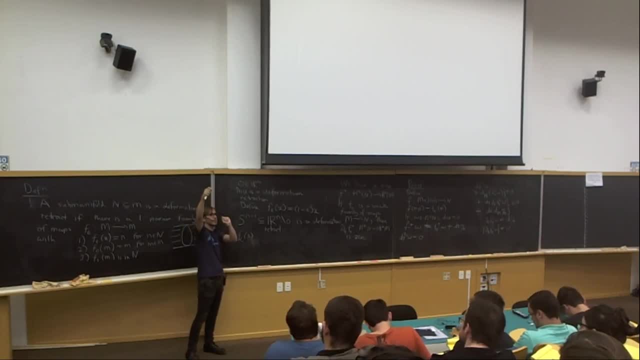 This is okay. And then how do I go down? I take one plus the multiplication retraction on this and I take the corresponding point on the sphere, which goes in the same direction, and just want to draw a straight line from one to the other. 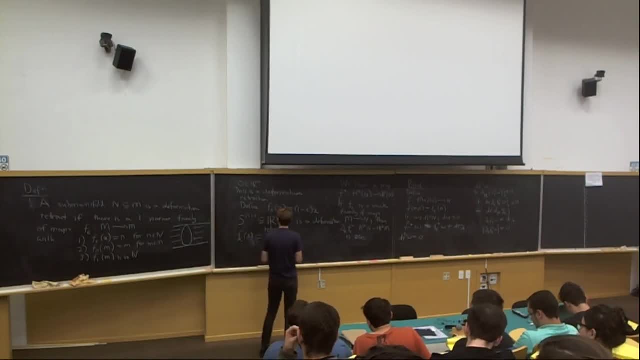 That's how I squish down. So the formula for that straight line it's t times x over the size of x, plus 1 minus t times x. So when t is 0, I just get back what I started with, and when t is 1.. 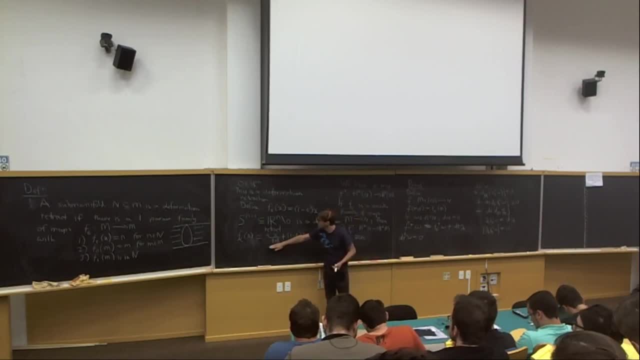 When t is 1,, this piece drops off and I get a vector on the sphere because this guy will have length 1, because I've divided by its length. So the reason for saying all this is if I have a deformation, retraction, then the cohomology. 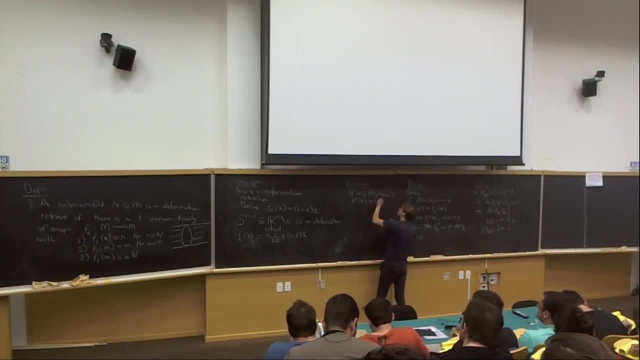 of n is equal to the cohomology of m. So all the cohomology classes really come from this essential topology which can't be removed. Here's the proof. We have this family of maps Now at the level of cohomology: f t star, from h k of m to h k of m. 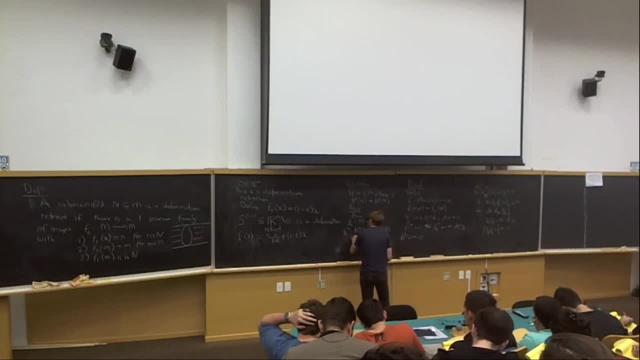 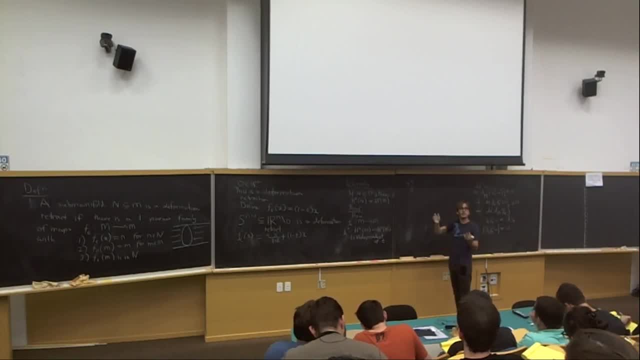 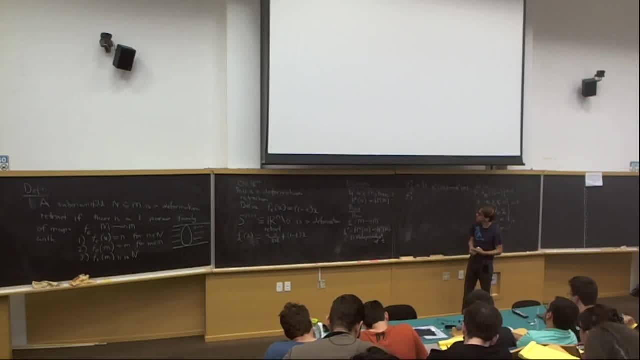 we're squishing everything down to n, So when it's 1. this map will factor through the map. So since these maps are the same, we're saying, well, whatever class we get here, it can't go to zero in the cohomology of n. 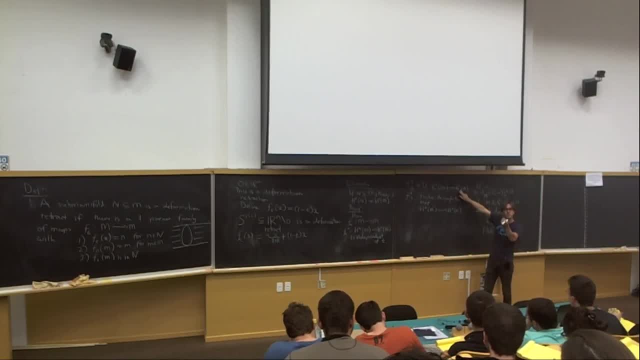 because if it did, it would go to zero when t was zero, which it doesn't. So this shows this map has no kernel and there's a similar argument that shows that it's onto. So I hope this wasn't. 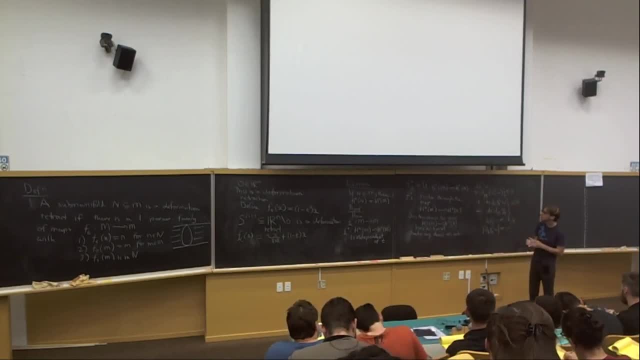 I feel this wasn't the clearest point. So the way to think about this argument is: the map, the pullback map in cohomology doesn't change when you vary it, so that's why I'm taking this map. So if I can squish everything down to this submanifold- 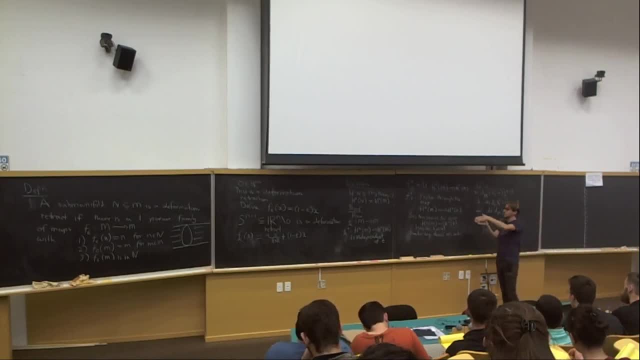 then all cohomology classes must come from that submanifold, because when a t was zero we see all cohomology classes, and when I go down we just see things coming from that submanifold. 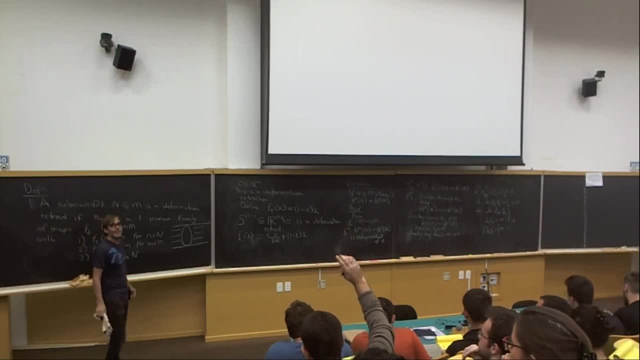 okay, yeah, of course sorry, thank you. yeah, sorry about that. everybody fit it in, but thank you. so. so this is good, because before we knew this we didn't really know very much about cohomology. we didn't even know that the 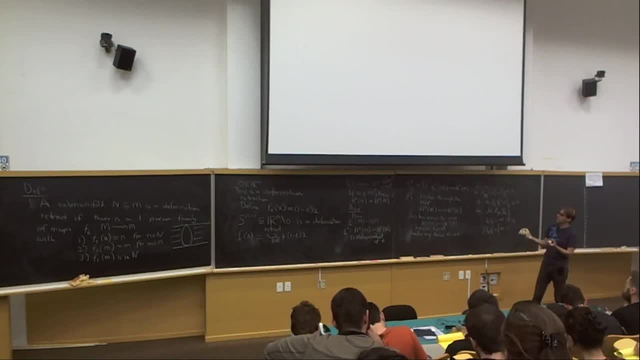 comb that the ball had no interest in cohomology. but now we know the cohomology can't tell the difference between a ball and a point. so now we can compute the cohomology of a ball. so this tells us the cohomology of: or n is equal to or if k is equal to 0 and 0 if k is not 0. 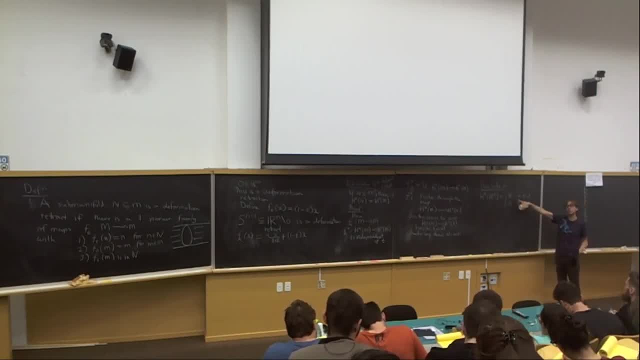 because this over here is the cohomology of a point. there's no interesting cohomology in or n. and it also tells us that, say, the cohomology of or n minus the origin is the same thing as the cohomology of the sphere. 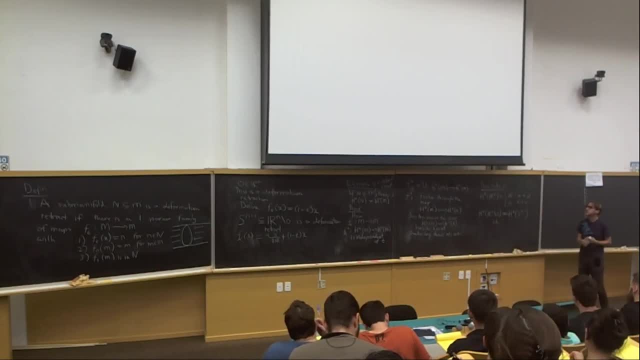 so the next thing we might try to do. if you wanted to pursue the computations of cohomology further, you could ask: how do we compute the cohomology of a circle? how do we compute the cohomology of a sphere? but after thinking about it, I've 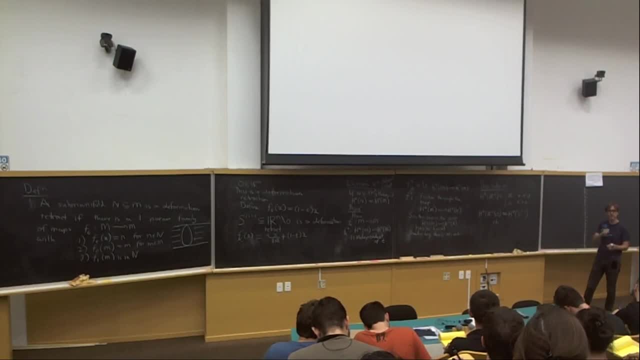 decided that it's just going to be too much to explain the methods to do this. there's a certain amount of algebra, and so I'll just I'll just give you the answers, and maybe some I'll give you the answers in one computational trick, which is useful. 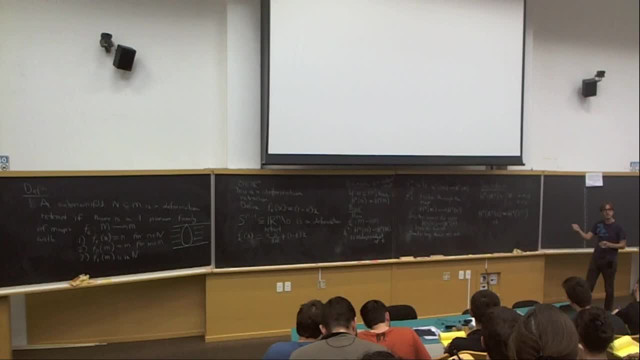 so this is the cohomology of a Depth of the sphere, and so what this means is take the correlation property and what this will take it to give you the alignment of the circle of the sphere and calculate. the сегодня's definition lasts a certain amount of. 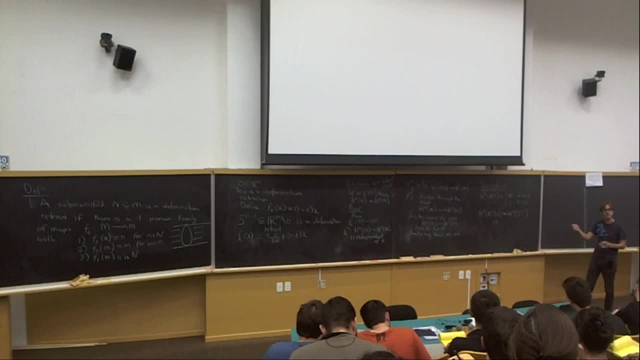 time, or if i is equal to zero, zero, if i is between zero and n, or if i is equal to n. Okay, so the intuition one has here, yeah, So there is a more general, i mean there's a slightly more general notion of like, being topologically equivalent, called homotopy equivalence. 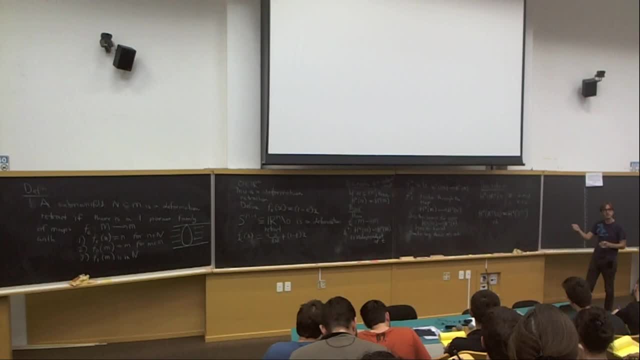 And cohomology is invariant. under that also, and the proof is basically the same, It just seemed easier to prove this case. What other equivalences were you thinking about, Like? what other operations were you thinking cohomology might be unchanged under? 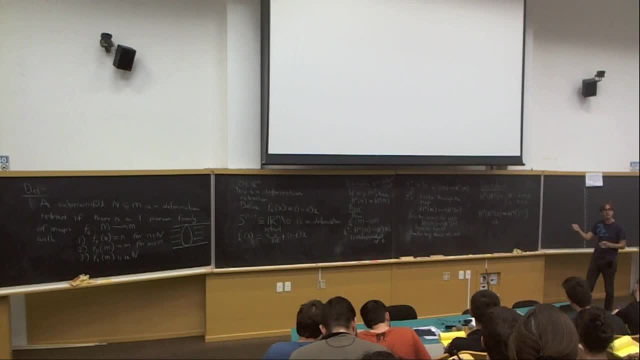 I don't know, it seems. I mean I sort of see your point. I mean, in practice, deformation, retraction is kind of good enough to get at the essence of having the same topology. So, in particular, you know we didn't say this, but our definition of cohomology didn't refer to any other struct. 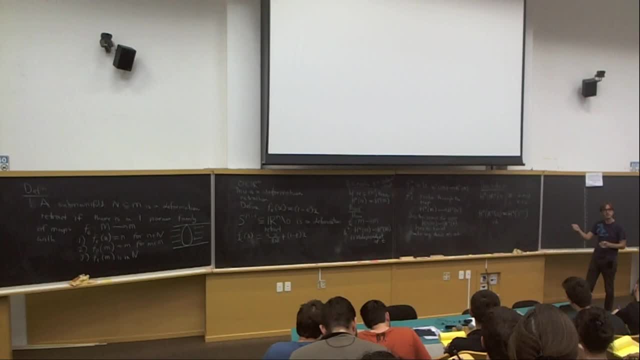 It was just it didn't refer to any way of measuring length on the manifold or anything like that, So it's already insensitive to like changing the shape of it. That was true from the beginning. So deformation retraction tells us a bit more. 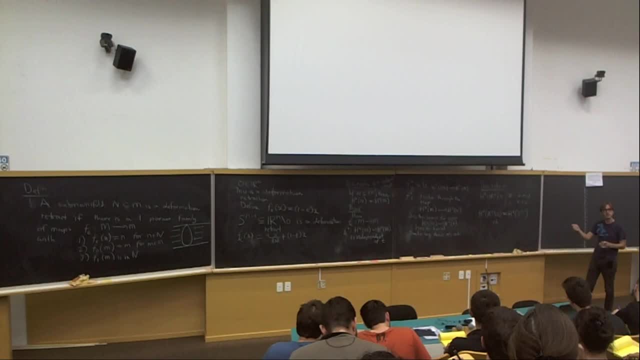 It's insensitive under making it a bit bigger in a kind of fuzzy way, which isn't Yeah, Yes, Yeah, I think I was really unclear at this point. Sorry about that, So maybe I'll do it over here, Okay. 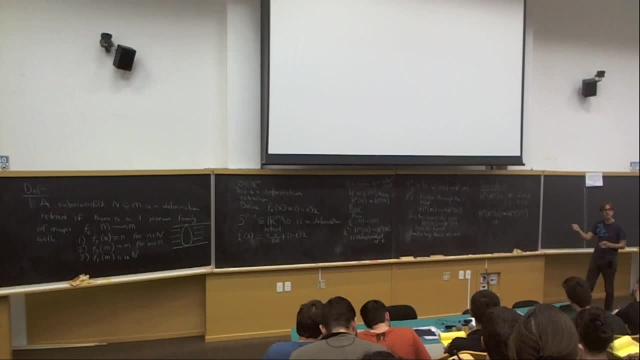 So F1. Is Maps everything down Down to N. So F1 is a map from M to M, but actually it lies in this subspace, N So F1 star Is a map. HKM, HKM. 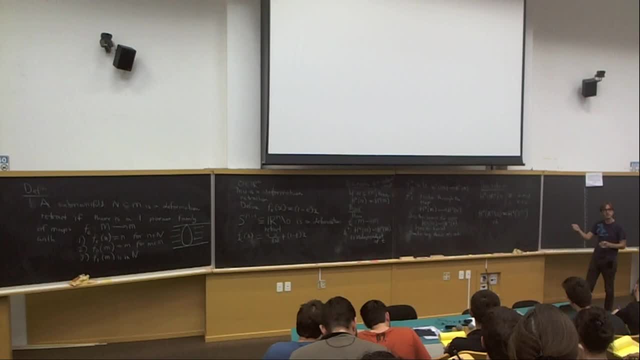 But It factors as, Just like F1 factors as squishing down to N and then including HKM To HKN To HKM, So this, So like we have some Mapping from here to here and it's written here, like you know, multiplying two matrices. 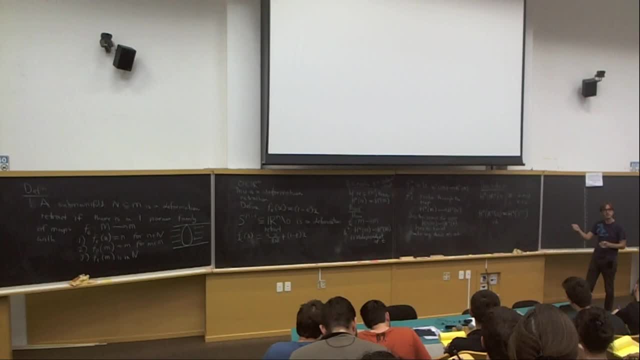 But we know That this composed map Is the identity map Because It, this composed map, doesn't change when I change the value of T. So a T equals zero was the identity map. So Now, if this operator had some kernel, 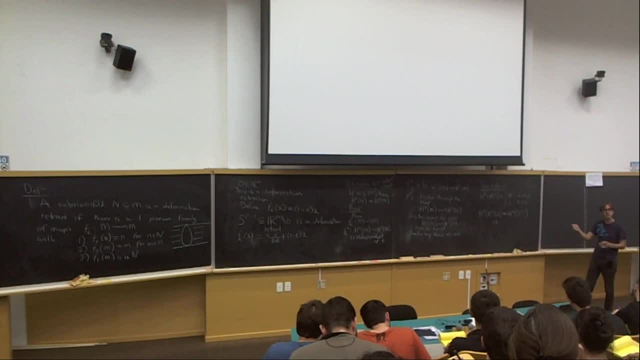 Then this composed operator also would have had a kernel And therefore the identity map would have had a kernel. But the identity map doesn't have a kernel. So that's how you know. Okay, Any other questions? Okay, Okay, Okay. 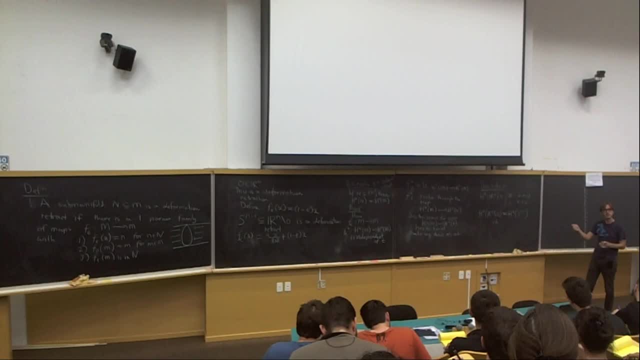 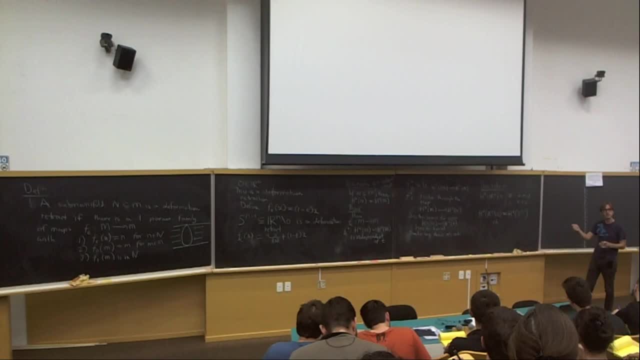 If I take the, the torus, The two-dimensional torus, And it's or when I 0.. Is two-dimensional: when I is one or when I is zero Is two, sorry. So the intuition here is that Taurus has these two cycles, one going that way and one going. 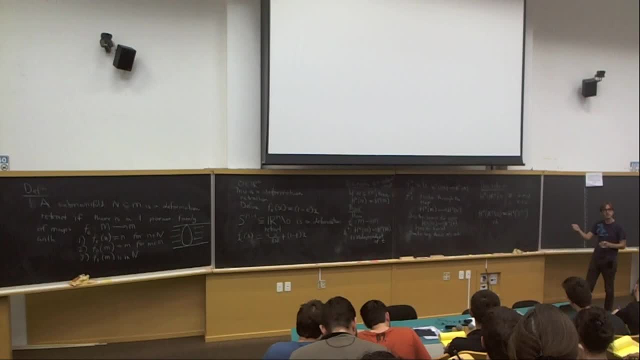 that way, Those two one-dimensional cycles are related to this two-dimensional space of cohomology in degree one You can write down: one forms d theta, d theta prime, whose integral around these cycles is two pi, And then there's a two-form and the constant zero-form. 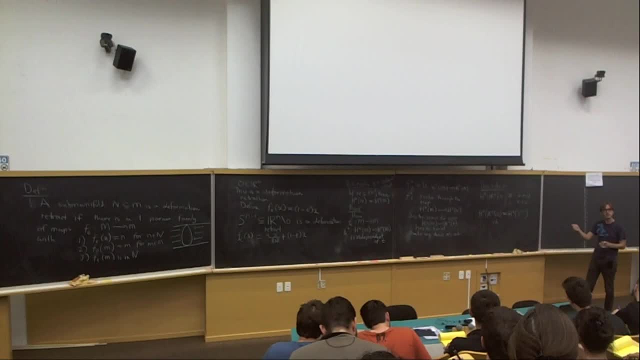 So, as I said, I've decided not to. I mean that the method for computing cohomology is called Meyer v Taurus sequence. Which is you take basically? 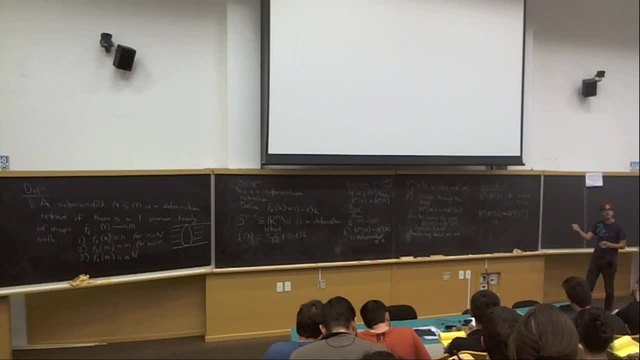 you take your space, you break it up into pieces and then you compute those pieces. could you speak a bit louder, sorry? 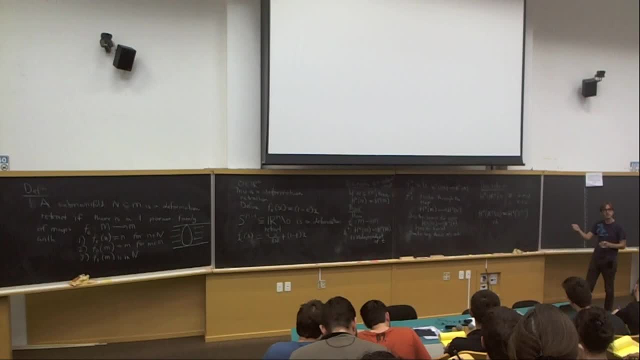 What's the physical meaning of it? So okay, so this: here we have this two-dimensional space. so I can ask, suppose I want to study solutions of the Yang-Mills equation which are massless, I mean which are like there is. you know, I have a four. 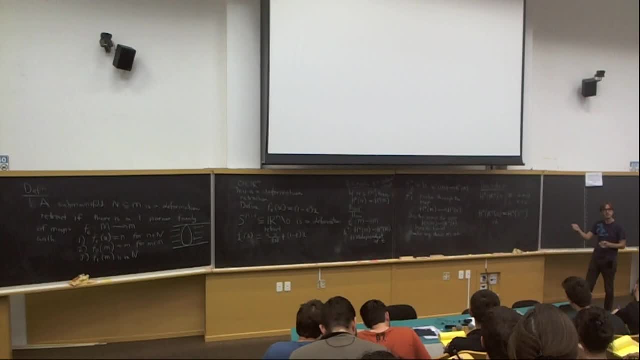 dimensional gauge theory on a torus, I took two compact directions. what are the zero modes? so this will be them there, you know. so these cohomology groups often have interpretations in those in terms of Kaluza-Klein reduction, for instance. was that the kind of thing you were? 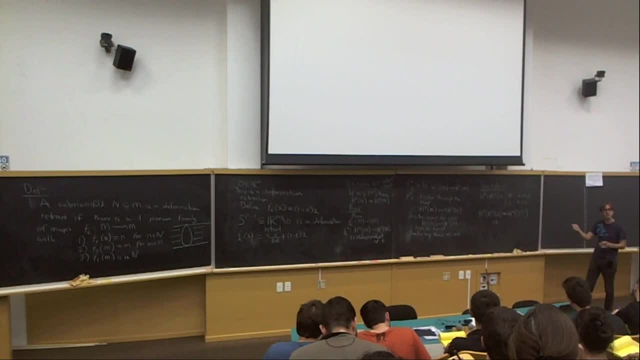 yes, so these, these, these cohomology groups for a three- well, I mean, these cohomology groups for a three groups have no reference. you know, their definition has no reference to physics. people came up with them because they wanted to study invariance, which will. 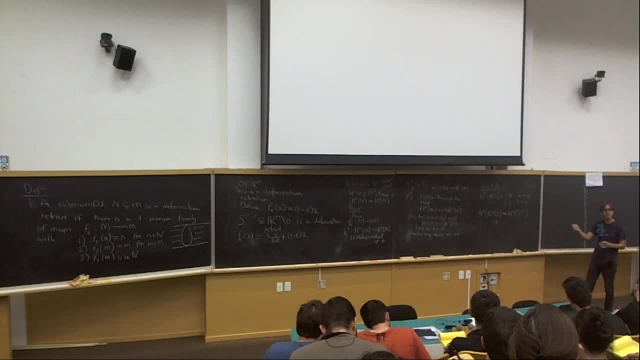 distinguish manifolds. they wanted to put precision on the intuition that the torus is two cycles. that's kind of. it's very easy to be hand wavy about these intuitions about how many cycles a manifold has. you have to be cohomology. 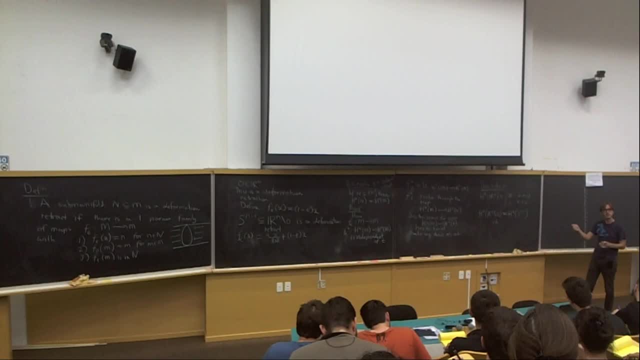 allows you to be precise about it, but they do have interpretations in physics. that's the intuitive interpretation of the answer that this cohomology is two-dimensional. there are physical setups where the RAM operator is the BRST operator, in which case you are computing what you said. 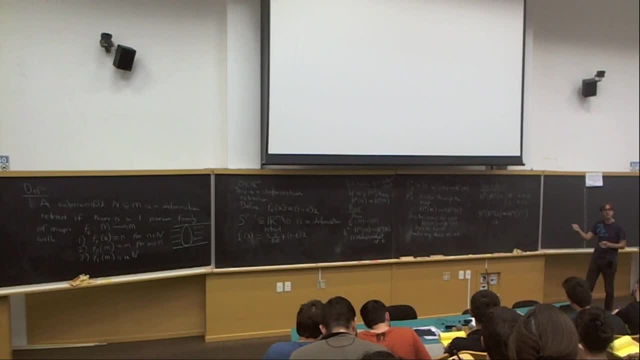 you. if you're interested in that, you can look at Whitney's paper on Morse theory from 1989. ok, so the final thing I wanted to say, but if you wanted to get a feeling for how to communicate cohomology groups, you know, there's some, there's some techniques. 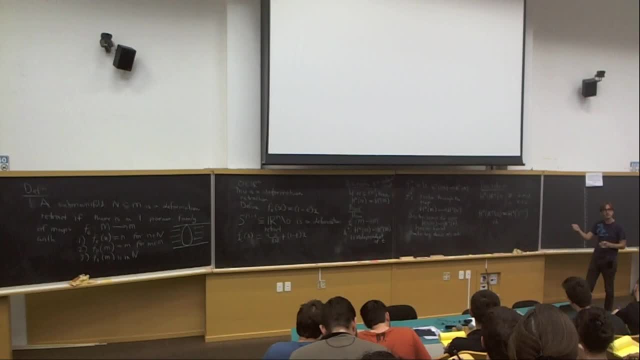 called the Mairi-Virtaurus sequence standard technique for doing it. but here's a here's a. Here's a useful rule. So if M is a manifold, you define the Euler characteristic of M to be the alternating sum of the dimensions of the cohomology. 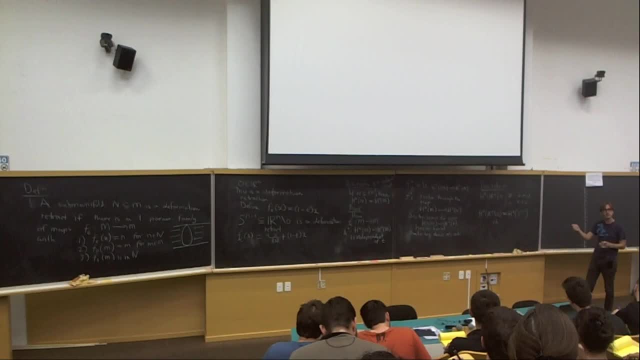 So it turns out by the Chern-Gauss-Benet theorem that this quantity is an average of the curvature of the manifold. If I have a manifold with no curvature, this quantity must be zero. Conversely, if I have a manifold for which this quantity is non-zero, then no matter. 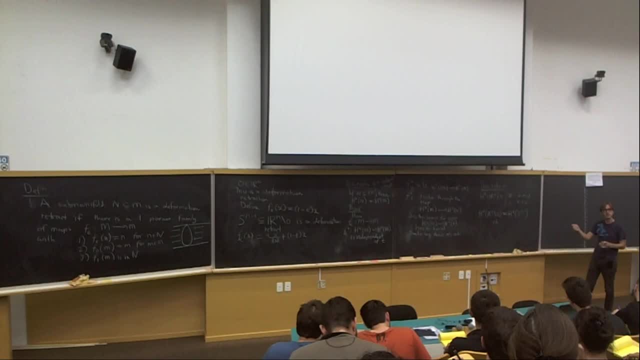 how I put a metric on it. there must be curvature somewhere. So the rule for calculating this is M, M. M is a union of two pieces. The Euler characteristic of M is that of U plus V minus that of the intersection. So with this you can play around and compute the Euler characteristic of various spaces. 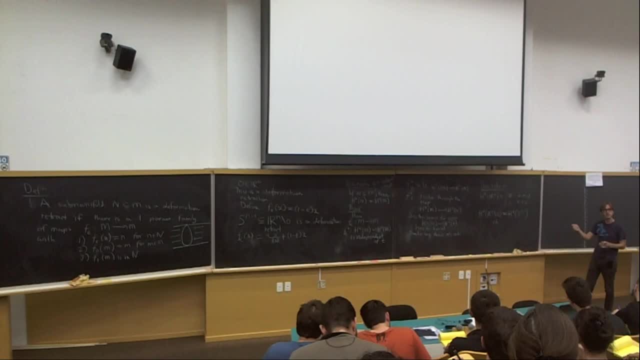 For example, the Euler characteristic of the N-sphere. The Euler characteristic of the N-sphere is 1 plus minus 1 to the N, and so on. Okay. 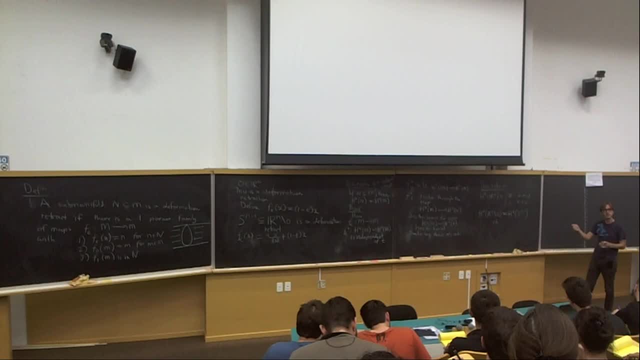 Well, let's say you're trying to compute the first comology of the plane compared to the first comology of the plane, with the points removed. 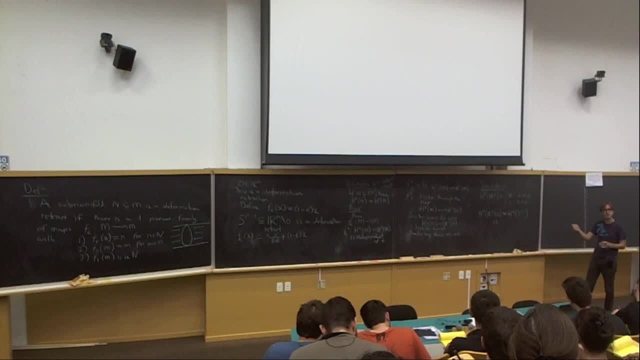 So on the plane at the point removed I could write 1 over Z, DZ and this is a closed 1-form on the plane with the point removed, but it has a pole at the origin, so it does not exist on the whole plane. 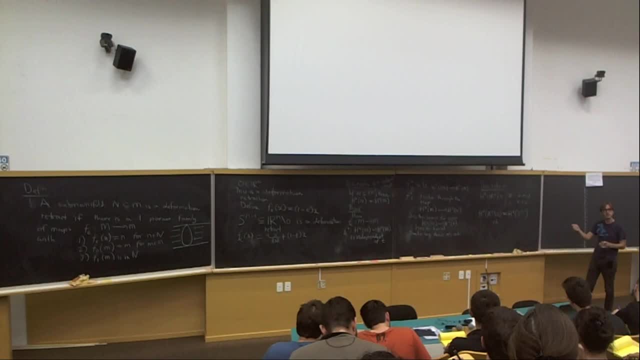 So that's the easiest way to see. Does that answer your question in any way? I mean, it is a bit subtle because locally everything is the same. So if you try to compute the differential equation in local coordinates, you're always. 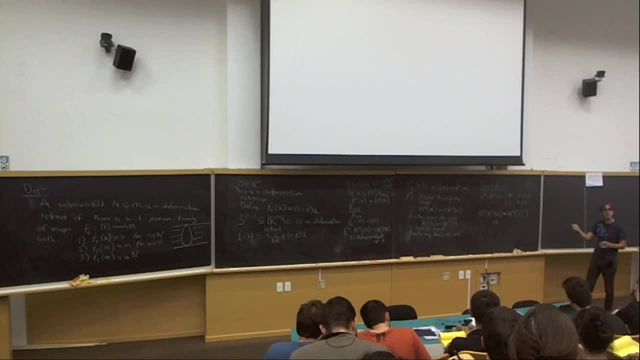 going to find the same answer. The reason why you define different answers globally is to do with patching these local pieces together. That is suppose you're trying to compute h1. Locally, every closed one form is d of something, So you might think: well, therefore, globally, 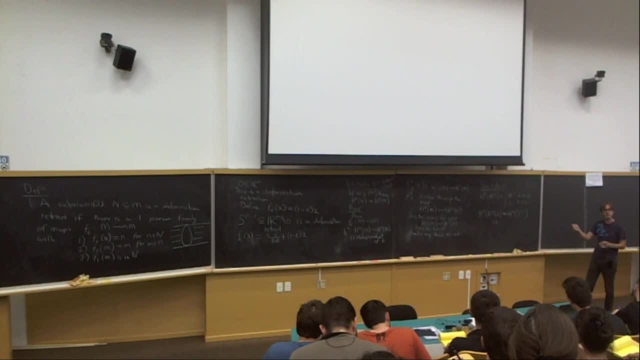 every closed one form must be d of something. But that's not true, because you try to patch together the things which it's d of and they don't quite patch. So here's the interpretation of this stuff in physics. So to get to the physical interpretation, 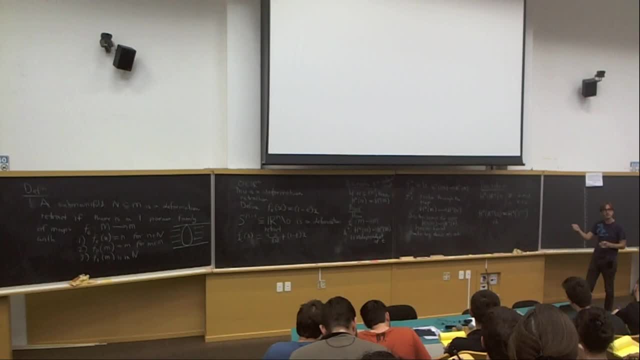 we need to define one more. We need one more operation which is called a Hodg-Starr operation. So this is an operation which depends on more than just the topology of m. It depends on actually how you measure distance And what it does is, it tells you. 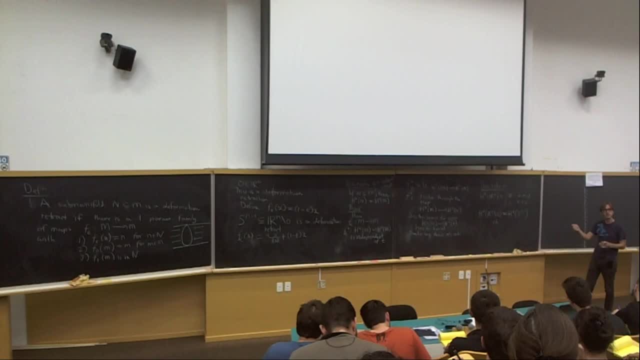 it takes a k form to an n minus k form, where n is the dimension And the formula in flat space star of dx, i1, dx ik is equal to epsilon i1 ik. j1 j n minus k. dx, j1 dx, j n minus k. there's a factor of 1 over n minus k, factorial, so it's 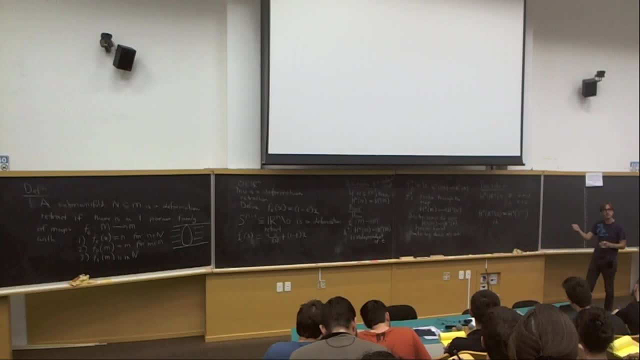 just some formula. but the thing you notice is, you know this, dx, i1 up to dx, ik misses some xi's and star of it picks up precisely the ones which this guy misses. so in dimension 4, which is the most important for our purposes, we have, for example, 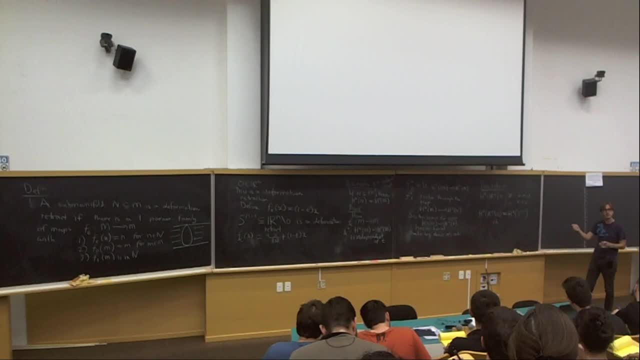 star of dx ii, which dx ii is equal to dx iii, which dx iv. star of dx ii, which dx iii is equal to minus dx ii, which dx iv and dx ii dx iv becomes. and here the minus sign is because 1, 3, 2, 4 is not quite secretly ordered. we have 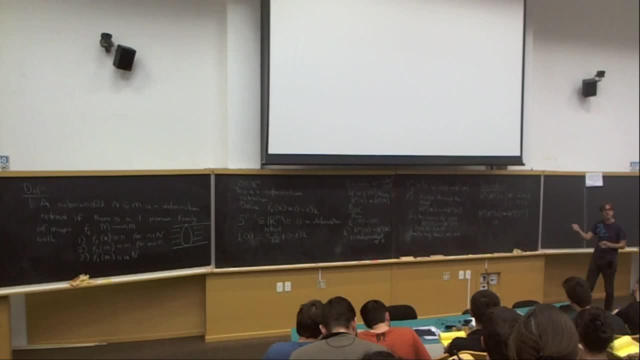 to switch the 3 and the 2 brings up a minus sign, and when n is 4 star, star is the identity. ok, so this seems to come out of nowhere. but the reason for introducing this operation is it gives a very slick way of writing down Maxwell's equations. 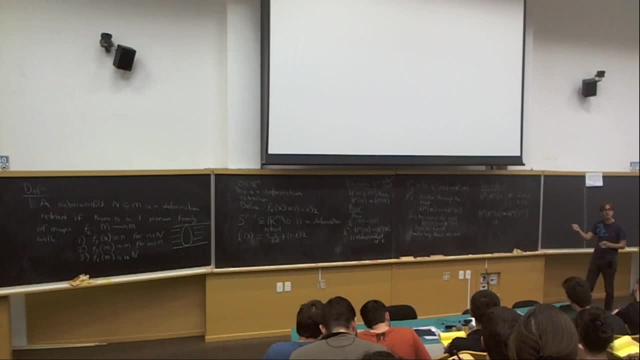 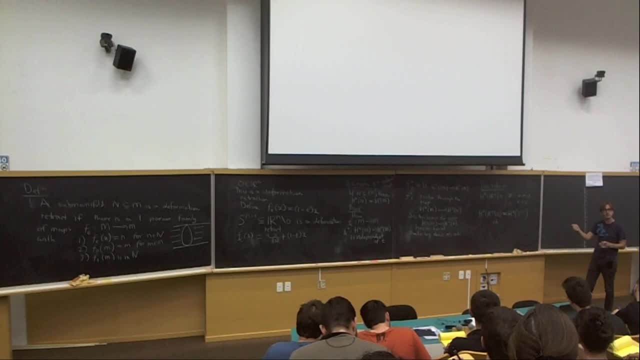 df equals 0, and d star f equals 0.. Okay, any questions? So if you really want you, can, you know, work in flat space and expand it out in coordinates and look at the bunch of equations that you would normally see? 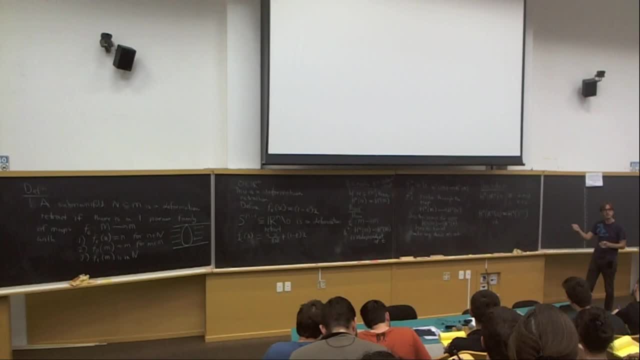 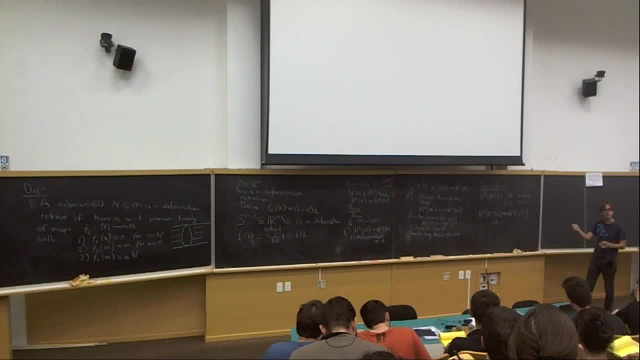 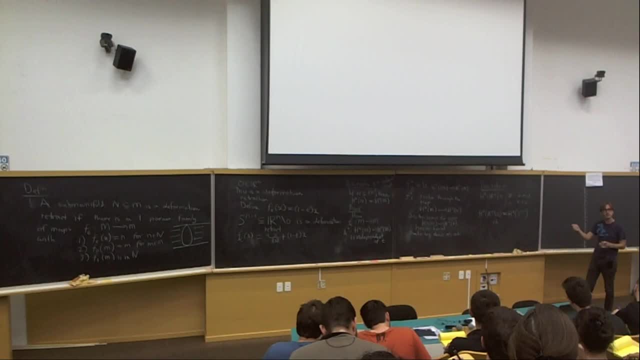 So it's So. that's one simple way. Yes, and you can see funny properties of electromagnetism because the space is a non-trivial topology. So normally if you work in flat space, this will not have an interesting cohomology class. 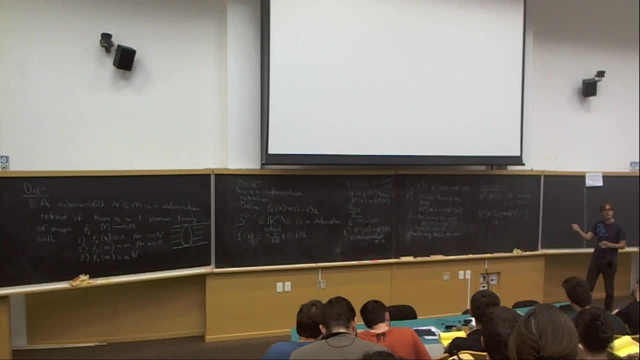 But if we're on something where I've removed a line from space, then this could have an interesting cohomology class And that's an interesting topological property of Maxwell's equation. With that, yes, I haven't. I mean there's a similar formulation- if I wanted to couple to a fermionic field, but I haven't done so. 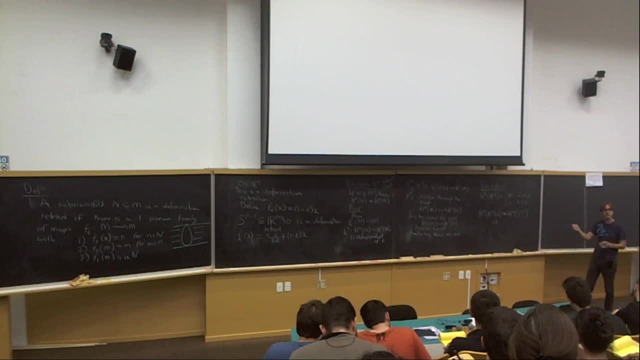 It's a bit more complicated. Okay, so if we have a surface in our manifold, then we can measure the integral over sigma of f and the integral over sigma of star f. So both of these, these are some very simple observables in the gauge theory. 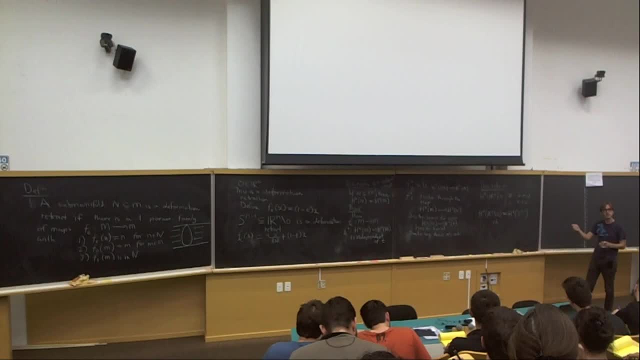 These are topological observables. They don't have a topological observable. They don't have a topological observable. But they don't depend on where I put the surface. They don't change if we vary the surface. So what this guy does is it measures. 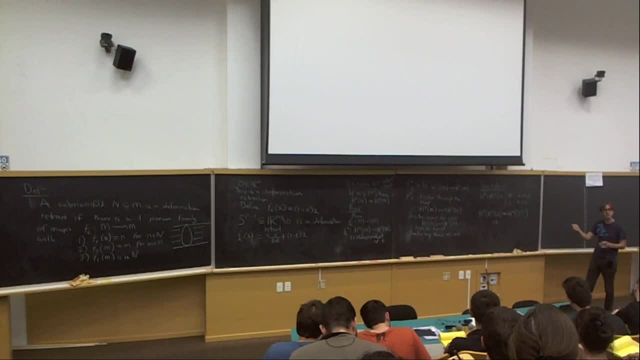 something like this, Something like the flux of the electric field, And this one is related to magnetic flux. and if I absolute lost the card real time and I'm just sitting here, Let's give you an example. I can take my field strength to be 1 over x1 squared plus x2 squared plus 3 squared. 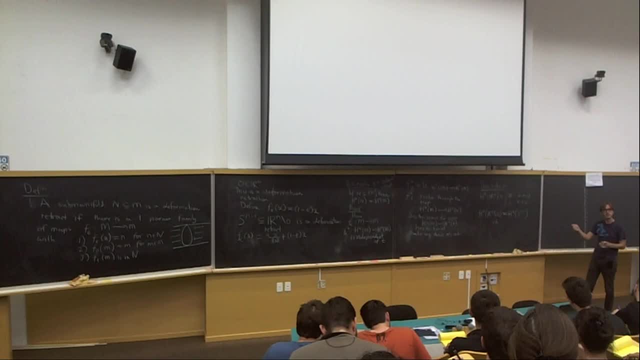 3 over 2, x1 dx1 dx2 minus x2 dx1 dx3 plus x3 dx1 dx2.. And you can check. In fact, I may have asked you to check. this was on the homework. I want this to be in four dimensions, so there's another dimension that it's closed. 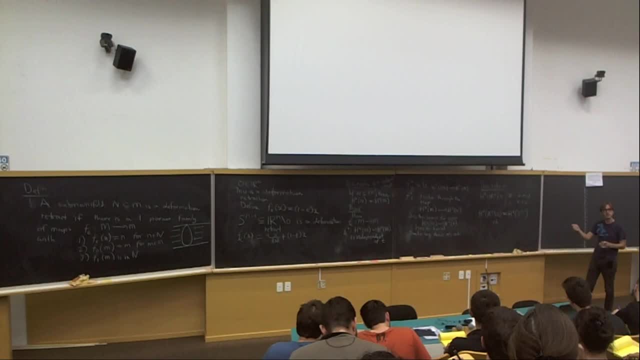 You can also calculate that star of f is 1 over x2 squared plus x3 squared half Times some x, i, d, x, i, y, h, d, t. Star of f: if you look at this equation going from here to here, you just have to do some manipulations with what star is. 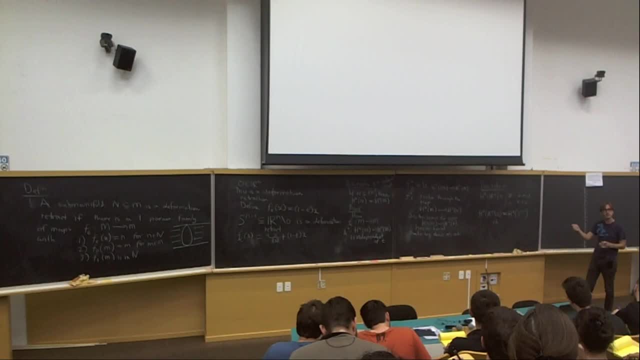 But if you look at this equation you'll see, well, some x i, d x i. that looks like it's applying the Dirac operator to something like this. This should be 3 over 2.. So that's as d of maybe minus d. 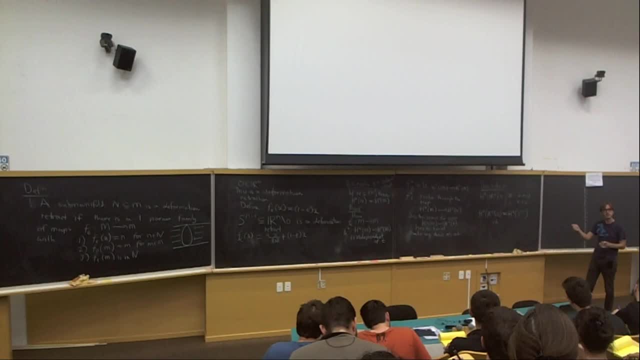 So because of this, you know, d squared is 0, so this equation implies that d star f equals 0. And that this f therefore solves Maxwell's equation, This one here. Thank you, yes, Sorry about that. 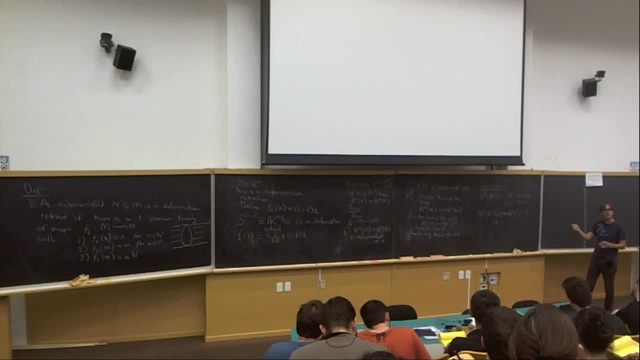 So this is So. this solution to Maxwell's equations is called the Dirac monopole. If I take the integral of this guy over the 2-Sphere, where the x is equal to 1, this is some constant, something like 2 pi. 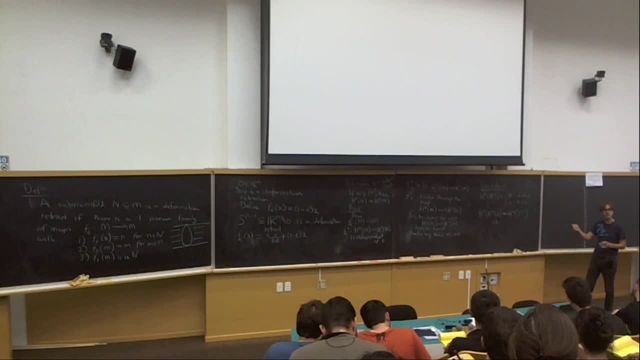 I don't remember the precise constant, butiller constant. so yeah, being a mathematician, I always get confused between electric and magnetic, because they are the same the equations. there's a symmetry, so that's not so yeah, so Dirac had some kind of an argument like this about magnetic. 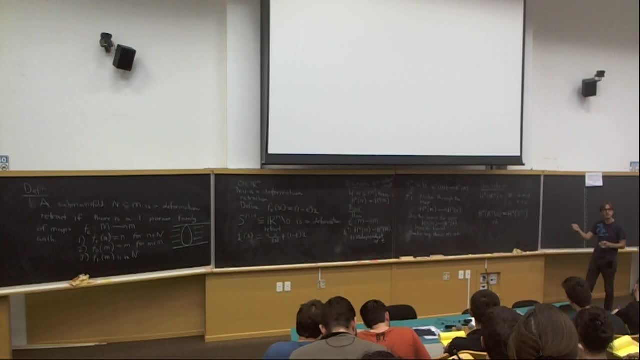 monopoles. I suppose this is the very simplest example of a solutions to Maxwell's equations which has an interesting topological property. I can, I can imagine, you know, I plug in this topological observable of the flux around the two sphere and it's not zero. 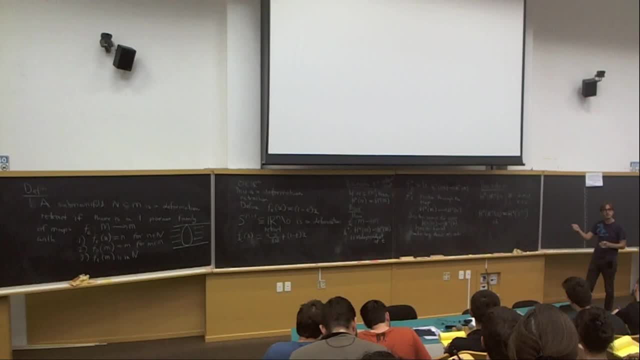 let's see what else. there's a few, a few other kind of kind of fun things one can do with that, with different differential forms and gauge theory. so let me- yeah, yeah, I'm see I'm gonna confuse you in between electric and magnetic at this point, so maybe, maybe, I. 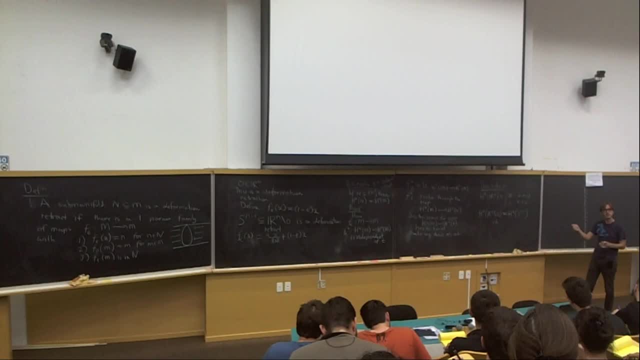 should have started with star F, but the equations are symmetric understanding after star F. so it's it's kind of a convention, what you call electric and magnetic poles. all right, so I'm going to go back to the question that was coming in. so the mains are two, invariance of two. 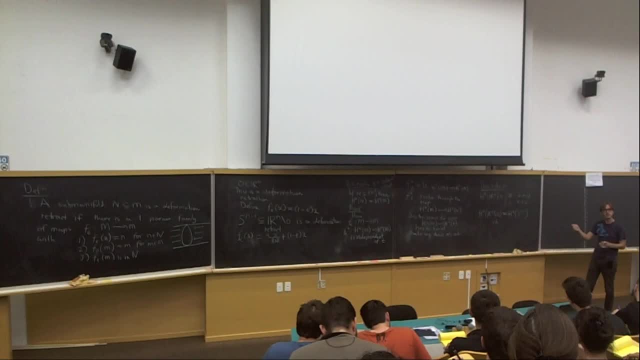 invariants at the top and one goes on to study none of you. yeah, so one we'll go. one goes on to study non of you. yeah, so to invariance that I can integrate over the whole manifold, So you can make an invariant that is even bigger or just smaller than the whole number. 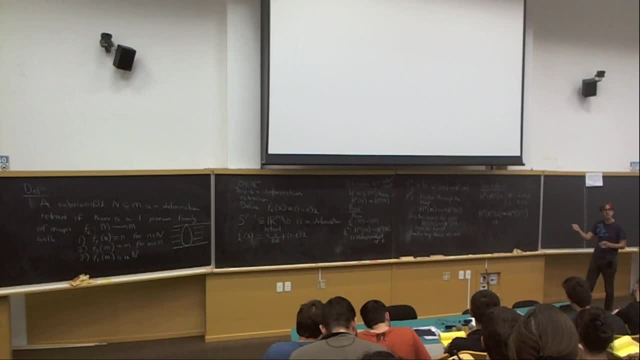 but you can make an invariant. that is here, and it's the only way to do that, but the whole number is too small like a scalar. yes, yeah, that's right. so there's, so that the. i think the two things you're thinking about are like f wedge star, wedge star f and f wedge f. 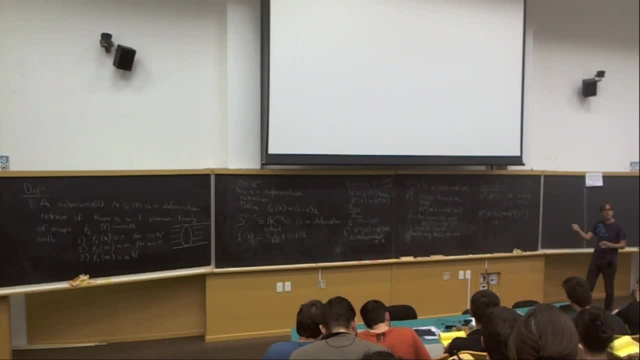 so this one, this one is the yang mills action and maxwell's equations are local minima of the integral of this action and this one it's sometimes called the theta angle and it's another measure of topological features. so so of the gauge field is that? is that your question? 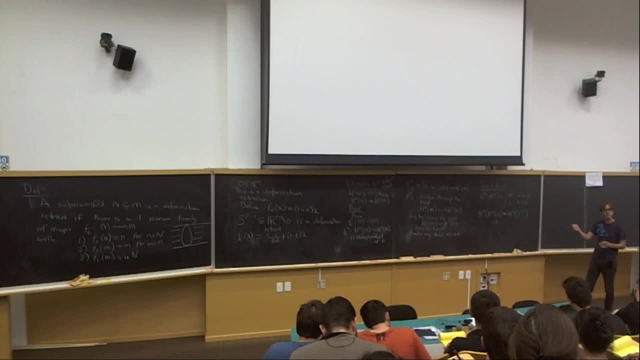 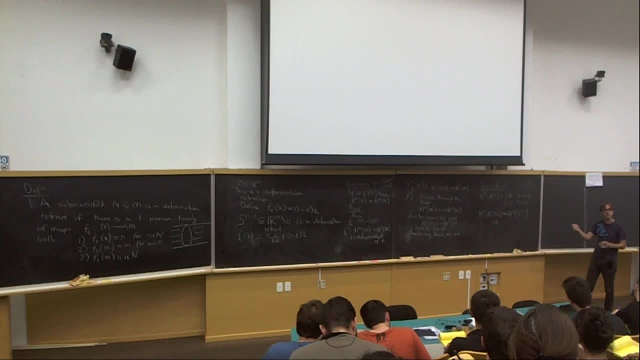 so so, so, so. so it's also fun to think about the electromagnetic potential. so so This is a one-form. A with dA equals F up to gauge equivalence: A plus A. A goes to A plus dEta, So the electromagnetic potential was of course something. 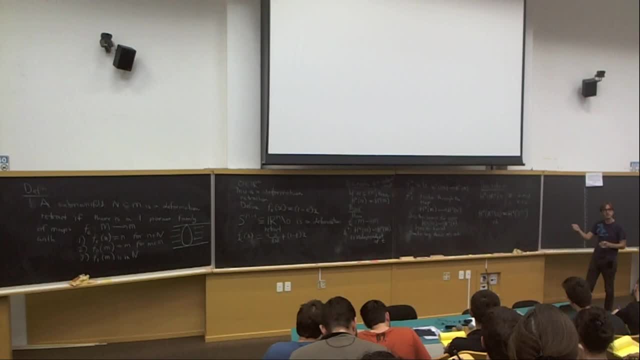 in the original formulation of Maxwell's equations. It was all about this guy, F, and he thought: oh, you know, sometimes we can write F in terms of A, where A is an auxiliary. It's an auxiliary, completely meaningless object. 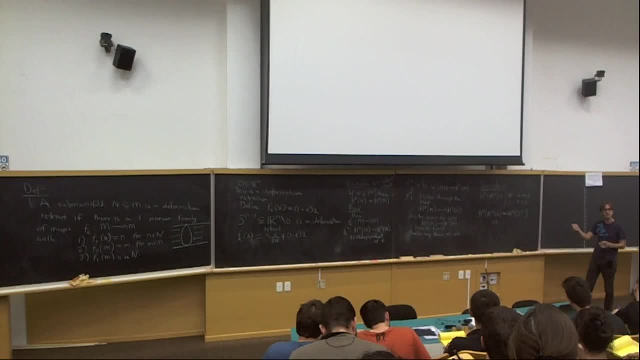 But later it was argued by Aronov-Bohm that actually A is kind of fundamental and has some meaning. So let me explain what they were doing as best I understand it, given that I'm not a physicist. So they study those A with 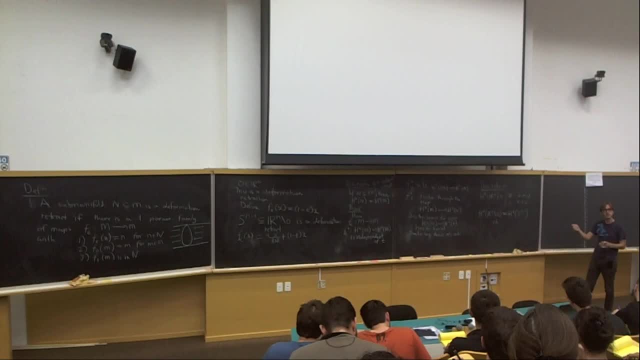 dA equals zero. So that means they have no field strength. And again, according to the original formulation of Maxwell's equations, studying these guys which have no field strength, well, you think the whole thing would be completely trivial, But it's not. 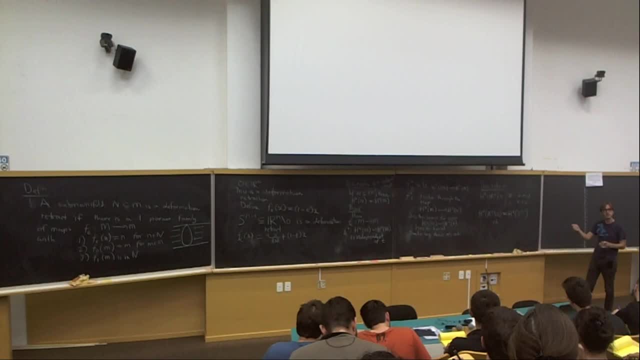 Now we already know what classifies, such As: There are classifications, There are classifications, There are classifications. There are closed 1-forms, modulo-D, modulo-gate transformations, which is adding on D of a zero form, So such As are the same thing as first cohomology classes. 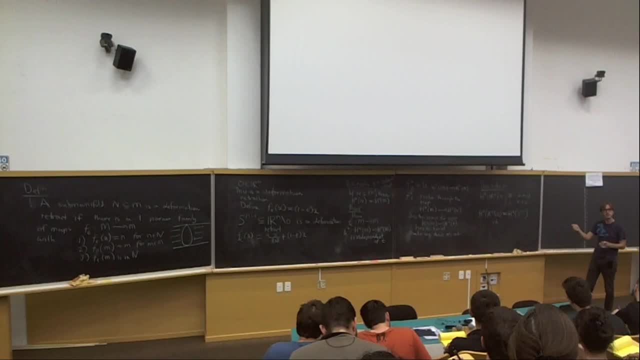 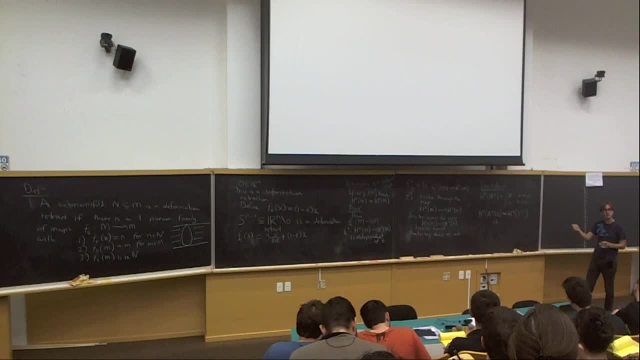 physics of this, better than me, will correct me if I make a mistake, when I make a mistake. So what's an example? So if space is or 3 minus a line, so I have this line removed, so maybe. so I'm not allowed to hit the. 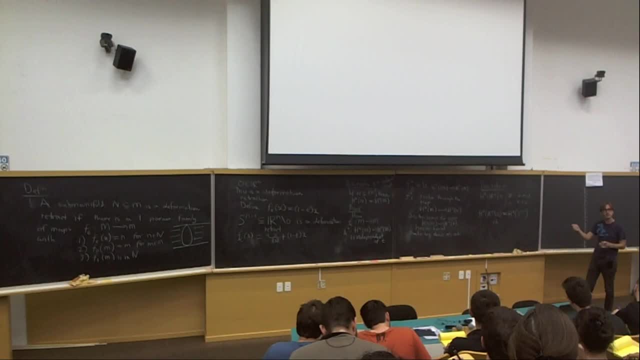 origin in the x1, x2 plane, then, well, intuitively, we can see that there should be some cycle right here. There's some cycle going around this line which can't be contracted. But we know a little more now and we have some feeling for cohomology. Well, space-time, 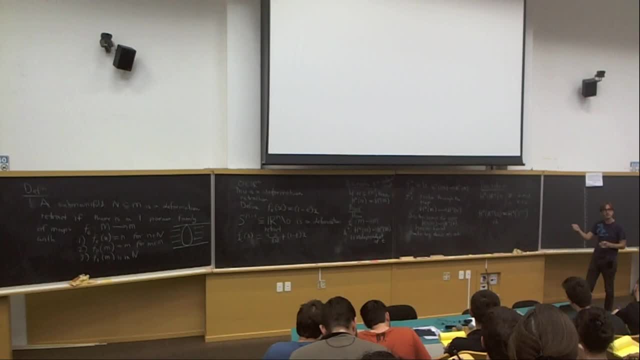 time, time time is or 4 minus a plane, and this deformation retracts onto a circle. By the arguments we had before, we can just squish everything down, but there's one part which can't be removed, which is this circle going around this line. 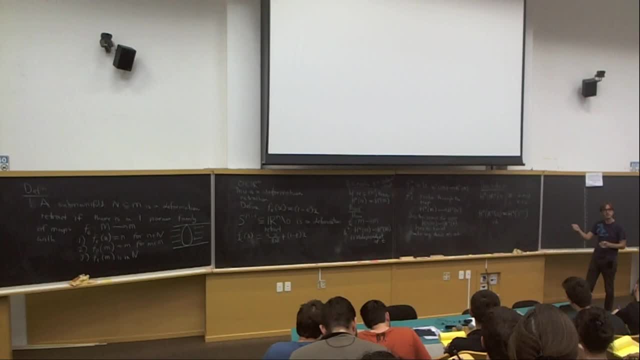 So now, of course, h1 of a circle is r, so h1 of space-time, and this will reduce shield. Pode G d- I started as a person, but guess what is also R? so that means there's some gauge field which is unique up to scale and up. 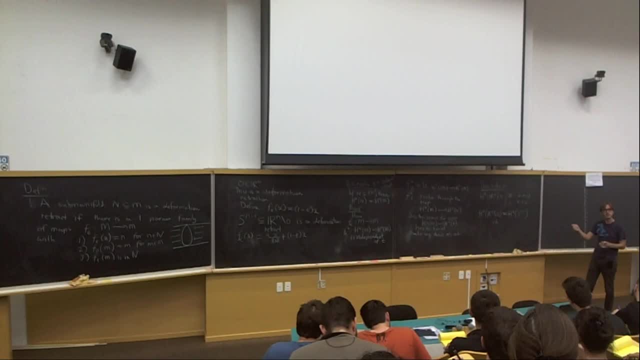 to gauge equivalence, which represents this cohomology class, and one way to write it is: it's 1 over x1 squared plus x2 squared, x1 dx2, minus x2 dx1.. Okay so next, Aronof and Bohm said: well, can we make some kind of measurement of this? 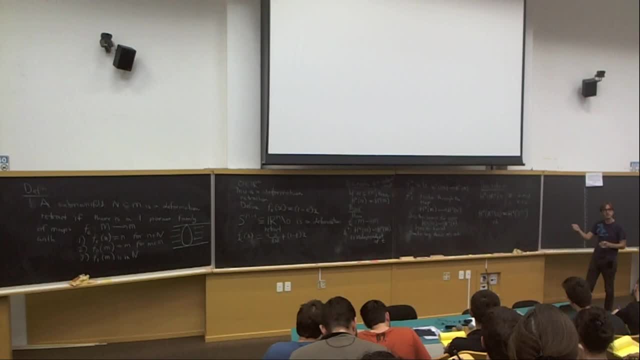 potential, this gauge field which is non-trivial even though it has non-trivial field strength. So what they did was they considered the integral around the circle of A and I think they had an exponential. So this is called a Wilson line. 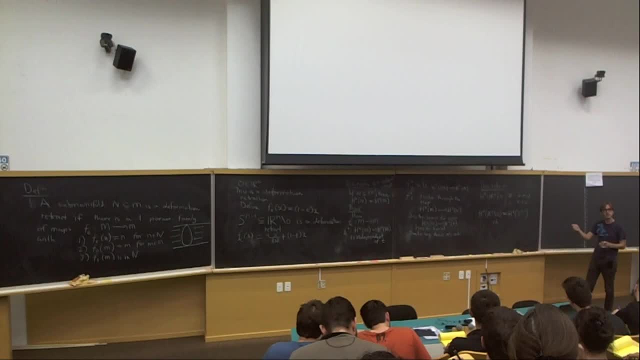 This is a special case of an operation which is very important in QCD. and what they said? well, their interpretation was that if we send a charged particle along the circle, Okay, so this is called a Wilson line. This is a special case of an operation which is very important in QCD. 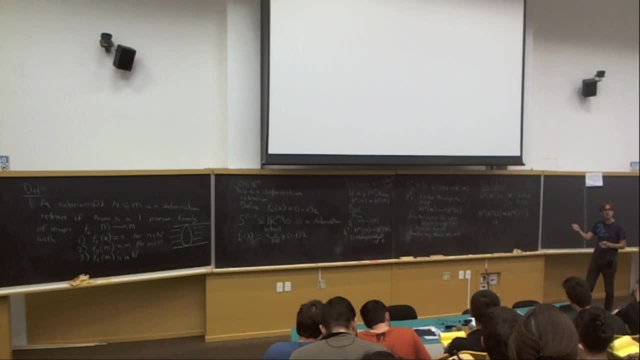 So the phase changes by this factor and, of course, precisely because A is a non-trivial cohomology class, we just SSed it. this factor is not equal to zero. it's some constant, maybe pi or something we can always. 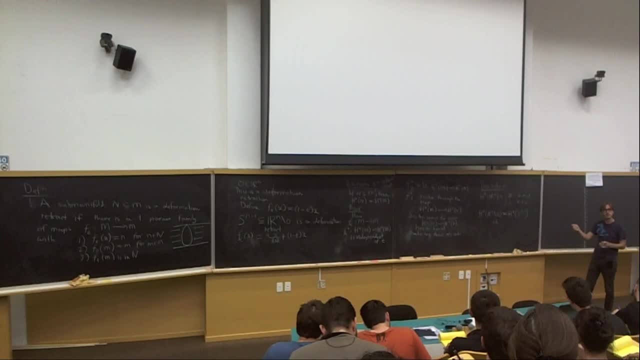 put in some constant here to adjust the value, so that this is really a measurable effect. So what other fun things can one do? So what other fun things can one do? So what other fun things can one do Out of time? and so I think this topic in physics, I think it really comes into its. 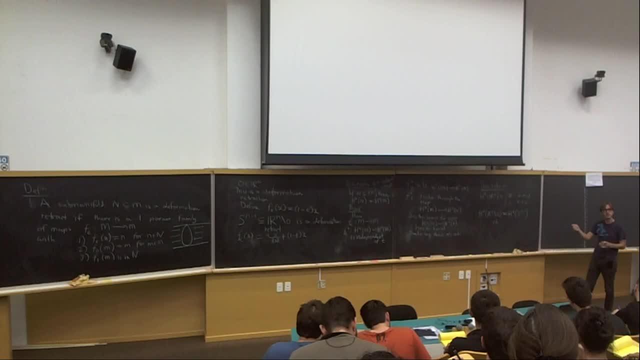 own in two areas, which is when you're studying string theory. you're not just talking about gauge fields. you might have fields which are forms of higher degrees, higher gauge fields, and instead of integrating them over a contour, you want to integrate them over. 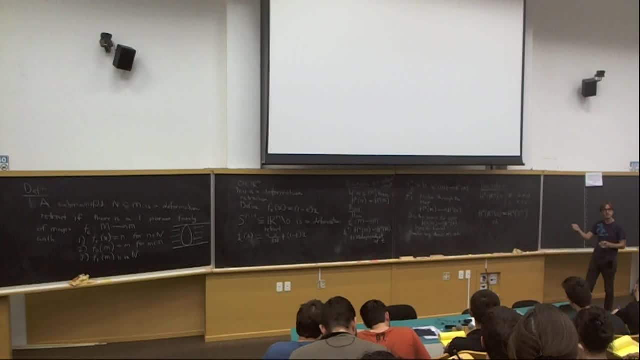 manifolds various dimensions. So then the language of cohomology is like a super useful language for understanding this story, And the other place where it's really useful is in an area I don't understand at all, which is the kind of topological methods in condensed matter. so I don't know much about this area. 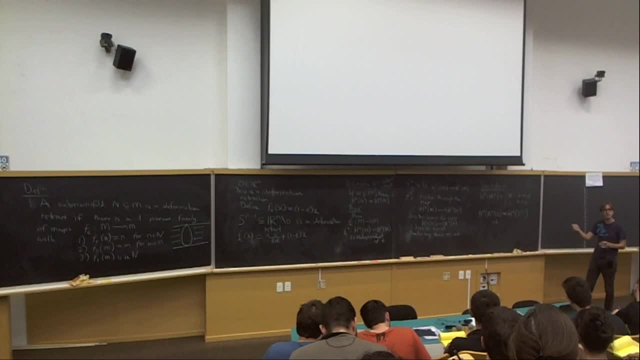 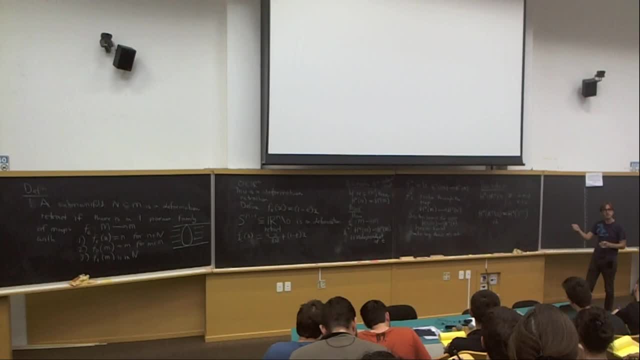 Questions. So don't wait until the next lecture, because this is his last lecture. I have one question about when you were doing the derivation for the homology classes of a product of m times the interval Mm-hm. I'm just wondering when you have two manifolds in general, 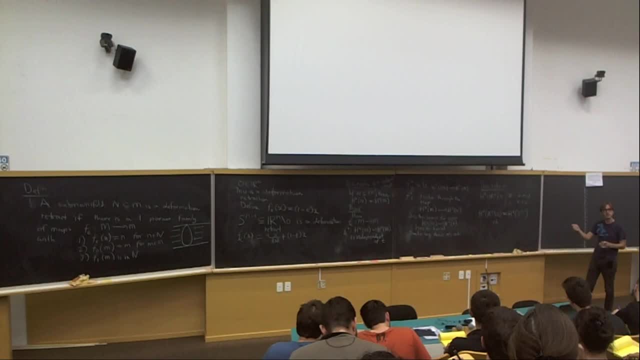 what's the rule to calculate the forms of the product of two manifolds? Is there any general result? or Well, I mean there is. So the rule is kind of for forms. it's easy to understand. You work in local coordinates. 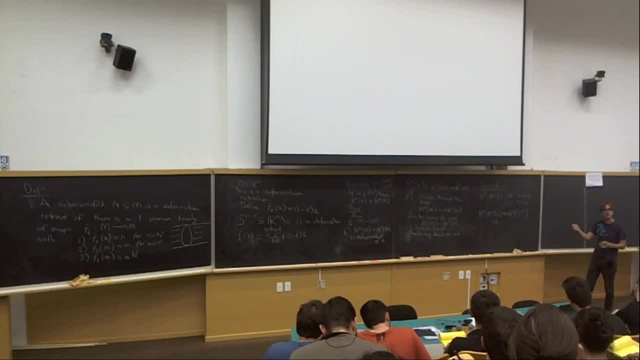 One is coordinates x, the other is coordinates y, And then a form is some product of dx's times, the product of dy's. that's it. So that's all it is. They're just something built up from some number of things on one side, and 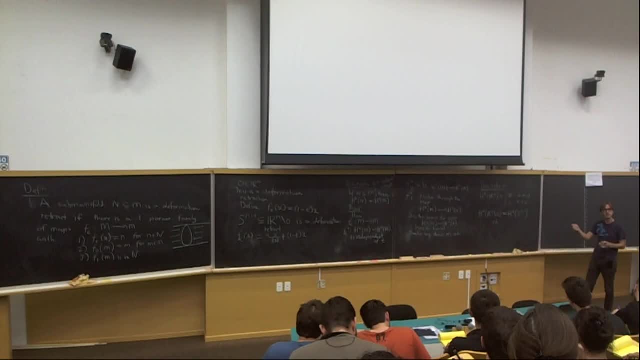 some number of things on the other side. So that's the reason why you write one form that does not depend on t and the other that depends on-. Yeah, exactly, Because on the interval it's either a zero form or it has a dt in it. 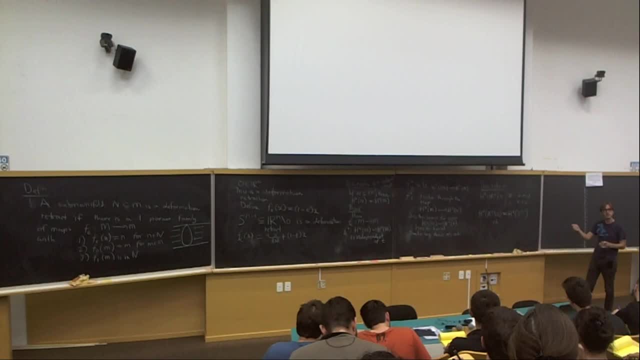 Yeah, it makes sense. Okay, and maybe one extra comment. When you talk about the solution to Maxwell equations, it's just a remark that this is only valid for this manifold, right? It's solution for this manifold where we were talking about in this example, right? 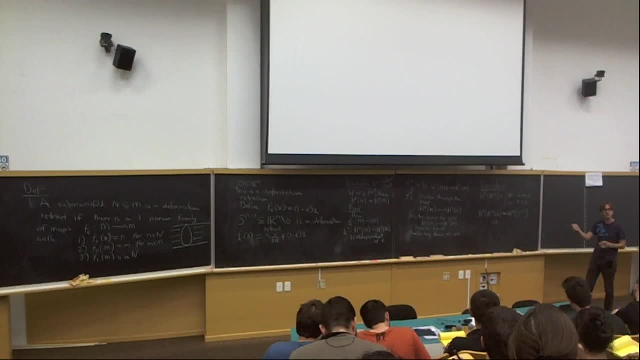 Yes, Yeah, we fix a manifold and we study Maxwell's equations on that manifold. Yeah, In the context of differential forms, what's the difference between space time and R4, the cause? No, none, there's no difference. And if you am doing Maxwell theory in curved space time,